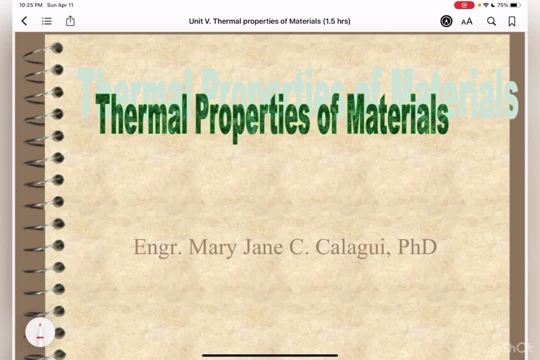 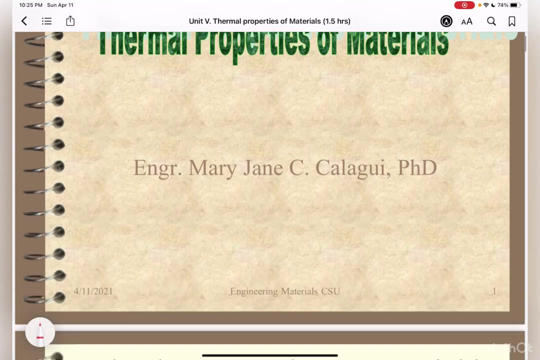 Though these properties can be found in your ever-reliable handbook, this can also be in some of your textbooks. Okay, so, in this lecture, we will focus on defining what heat capacity is, specific heat, thermal expansion and thermal conductivity, which are often critical in the practical utilization of solids. 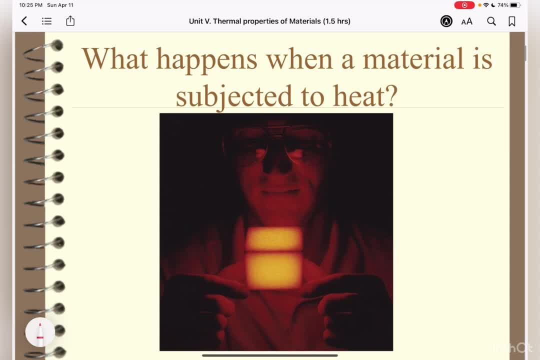 So, to begin with, let's take a look at this photograph. What happens when a material is subjected to heat? Of course, the usual answer to that is: it becomes hotter. Now this photograph shows a white cube, A white cube of silica fiber. so this one which, only seconds after having been removed from a hot surface, can be held with the bare hands. 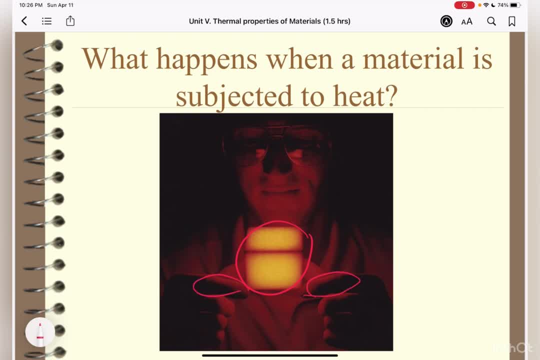 Take a look at this man. He's actually holding that silica cube. So what transpired here Initially? the heat transfer from the surface is relatively rapid. However, the thermal conductivity of this material is so small that heat conduction from the interior from here. 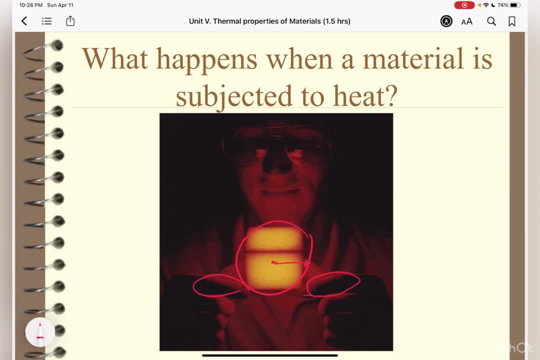 going to the exterior is very, very small. So the maximum temperature is approximately at 1,250,. but take a look, it can be held by a bare hand because, as I've said a while back, the thermal conductivity is so small. 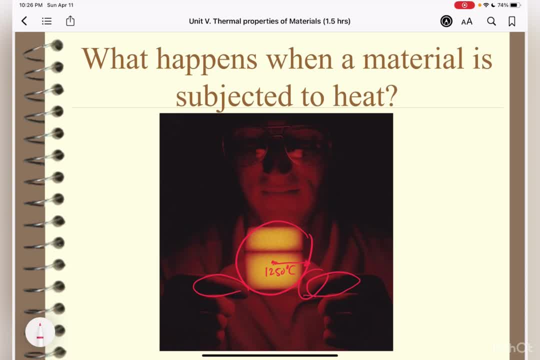 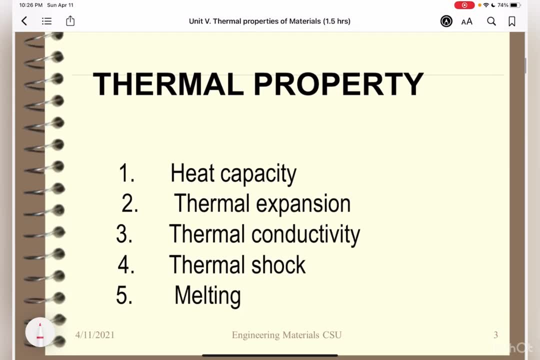 The heat conduction from the interior to the exterior is so slow. Okay, so the topics for this lecture is about thermal property. When we say thermal property, it means the response of a material to the application of heat. So definitely, this is response of a material to the application of heat. 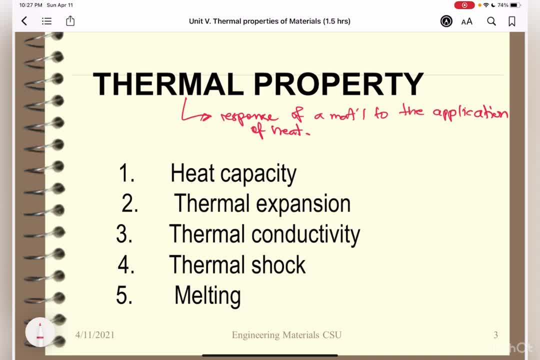 So a solid absorbs energy in the form of heat, It's thermal Temperature rises and its dimensions increase. The energy may be transported to a cooler region of the specimen if temperature gradient exists, and ultimately the specimen may melt. So we have to deal with the different properties, such as heat capacity, thermal expansion, thermal conductivity, thermal shock and, last but not least, is melting. 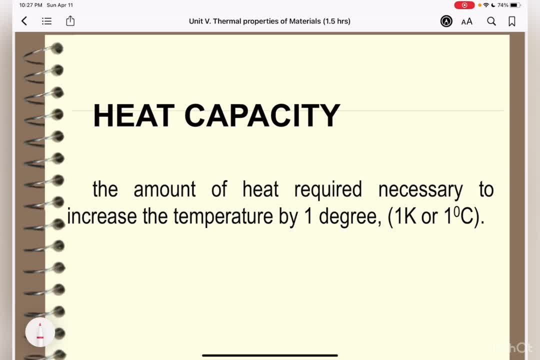 Okay, to begin with let's define what a heat capacity is. From the definition From the book. it is the amount of heat required, necessary to increase the temperature by one degree. So a solid material, when heated, experiences an increase in temperature, signifying that some energy has been absorbed. 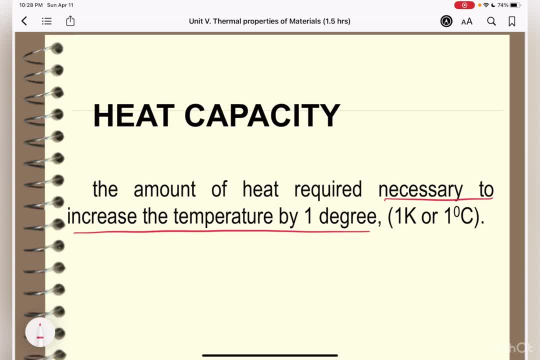 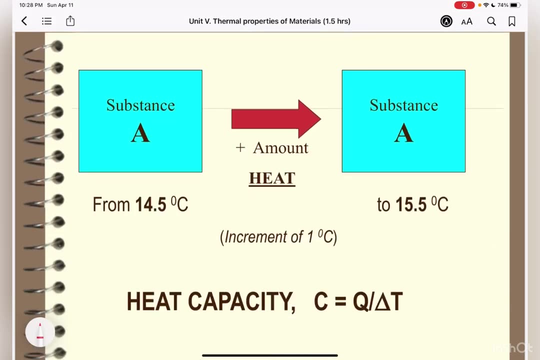 So heat capacity represents the quantity of heat required to produce a unit rise, So one degree, one Kelvin or one degree C in temperature for one mole of a substance. So like, for example, if I have one mole, Like, for example, if I have substance A, the amount of heat to raise, say, the original temperature, is 14.5 degrees Celsius. 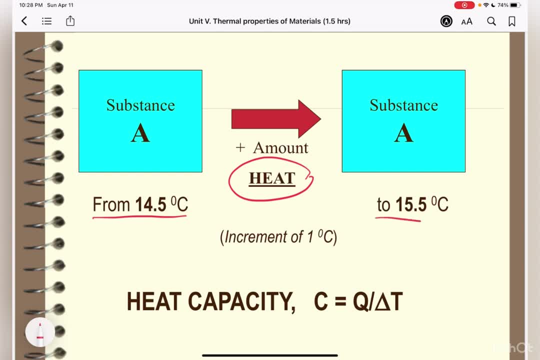 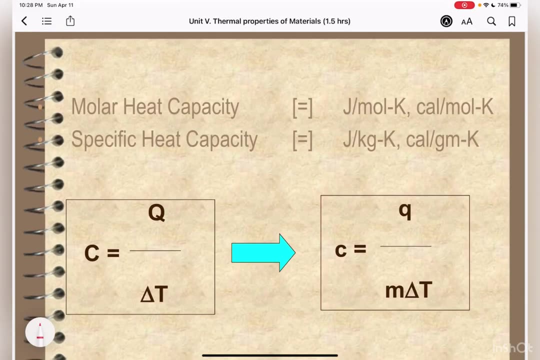 The amount of heat to raise the temperature to around 15.5 is what we call heat capacity, given by the equation C, is Q over delta T. Okay, so as not to confuse, note the difference between a molar heat capacity and specific heat. 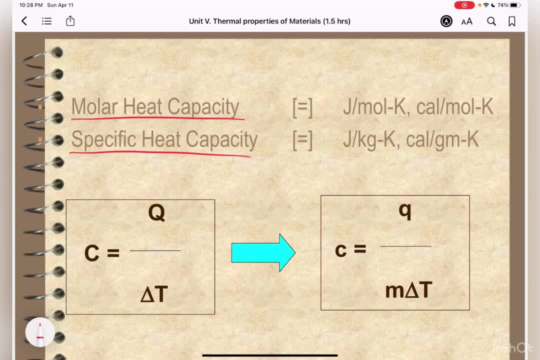 So when we say, if it is the amount of heat needed to produce one degree rise in temperature per mole of a substance, it is what we call a sure heat capacity. It has a unit of joules per mole Kelvin or calories per mole Kelvin. 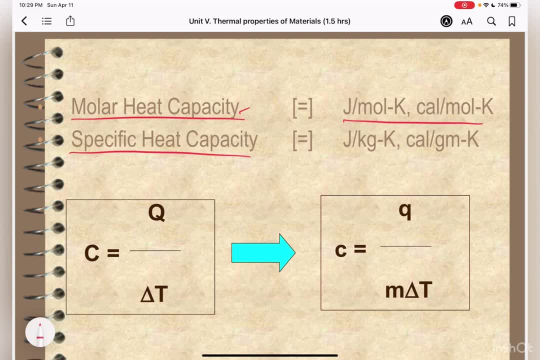 However, specific heat represents the heat capacity per unit mass, Or sometimes it is in small c. Some of the books uses it. So there are two ways in which this property may be measured, according to the environmental conditions accompanying the transfer of heat. One is the heat capacity while maintaining the external pressure, what we call as your Cp. 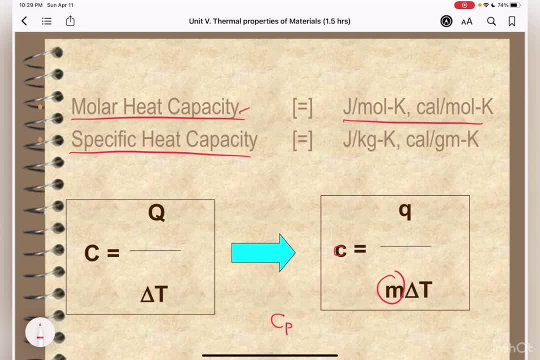 And the other is, of course, the heat capacity at constant specimen volume, or that is Cv. I think you're familiar with this already from chem or thermodynamics, So you have learned this: that Cp is always greater in magnitude than Cv. 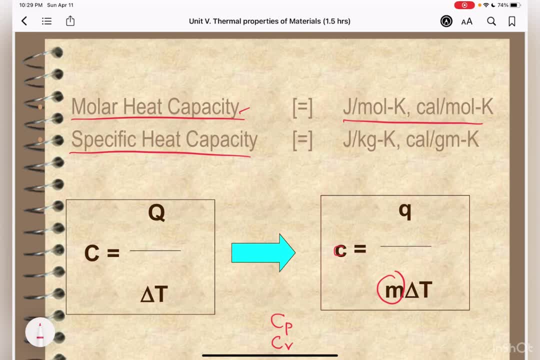 but very slight difference for most solids at room temperature and at below room temperature. So you would know that generally Cp is greater than Cv, But for most solids Cp is almost equivalent to Cv. This only acts at room temp and below for most solids. 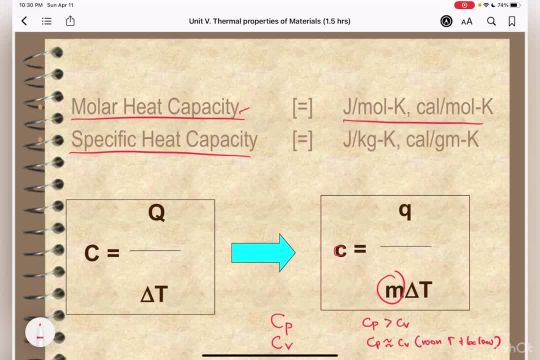 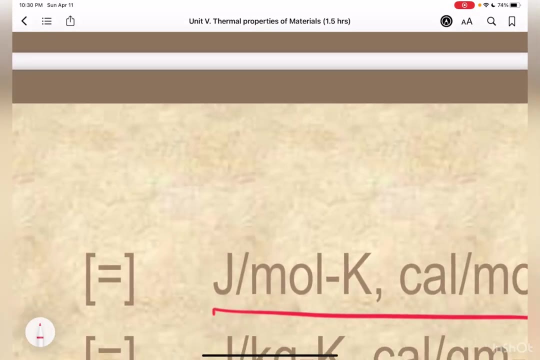 Okay, Now let's examine the relationship between Cp and Cv, The relationship between the heat capacity at constant pressure and heat capacity at constant volume. Note that from our equation, Q is equal to Nc delta T. we can get a constant pressure to be Q at constant P would be Ncp delta T. 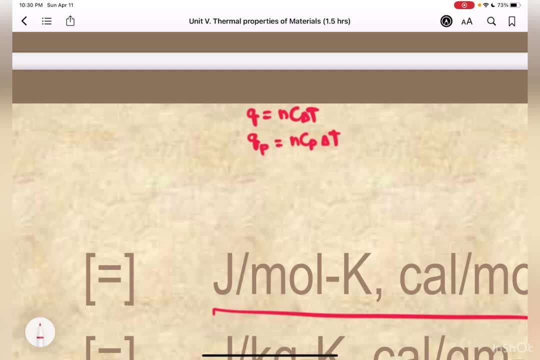 Okay, So this value is exactly the same as the change in enthalpy, So this can be also equivalent to your delta H. Now, at constant volume Qv, which is also equivalent to Ncv delta T, this is exactly equal to the change in internal energy, or that's your delta U. 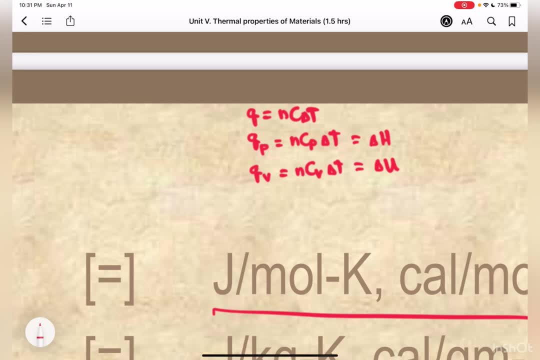 And we know that by the molar heat capacity, that when N is equal to 1, this is for an ideal gas. you would know that if I would equate that delta H is actually equal to delta U, review your thermodynamics plus delta Pv. 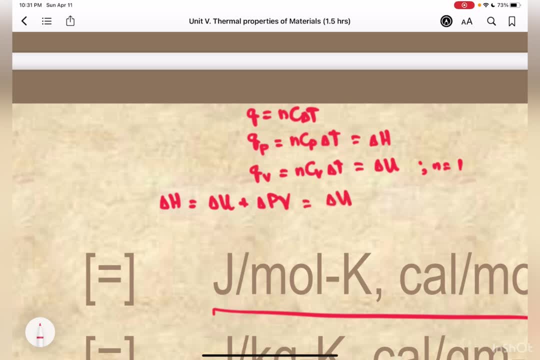 Or ideal gas. that is delta U plus delta Pv is R. Okay, Pv is R times T, right? This one Pv That's equivalent to your RT. Therefore, if I am to equate delta H, you know that it's delta U. 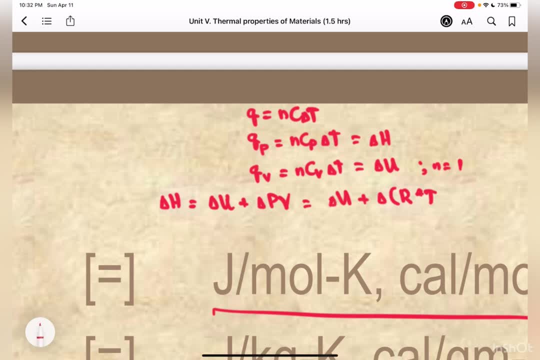 Sorry for that. It's delta U R times T And by substituting therefore the values for here delta H. so if I am to use delta H to be Ncp delta T, that is equivalent to your delta U plus delta T R multiplied by T. 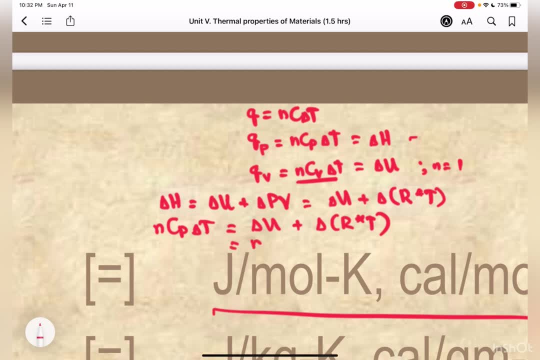 Or delta U is actually Ncv. delta T plus R is constant, so that is R times delta T. Finally, for one mole of substance- you know that this could become this is canceled. so Ncp, delta T over N, So this becomes Cp is equal to. 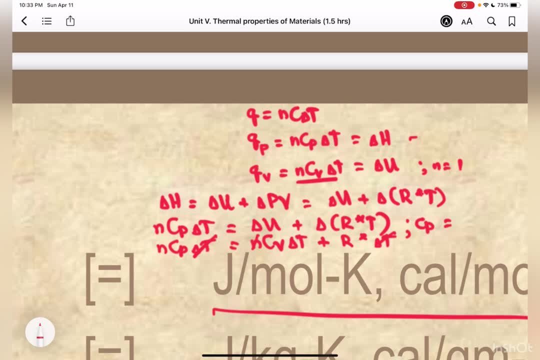 so the delta T is also canceled. Cv plus R, Or right In thermodynamics, Cp minus Cv is equal to R. So that's how we arrive at the equation, or this is the derivation of the equation, for the relationship between the heat capacity at constant pressure. 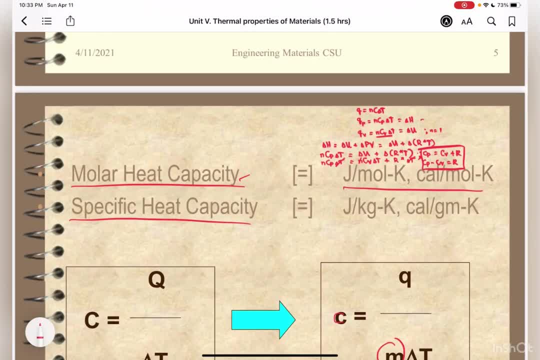 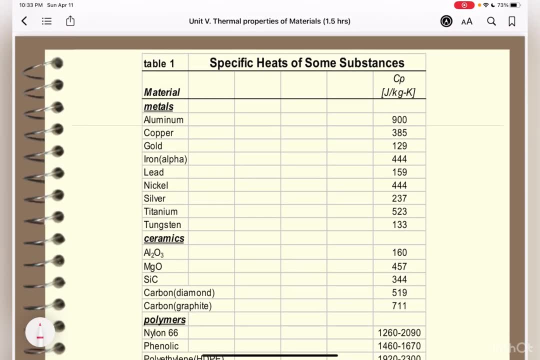 and heat capacity at constant volume. Okay, Now I have here a list of the specific heat of some substances listed. So some of the metals would have very high Cp: ceramics and then polymers, Okay, So take a look at this figure here. 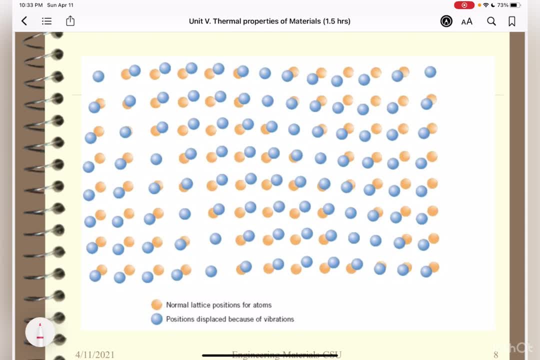 So in mole solids the principal mode of thermal energy assimilation is by the increase in vibrational energy of the atom. So these vibrations are coordinated in such a way that the traveling lattice will So take a look. If the normal position of the lattice is given by the orange. 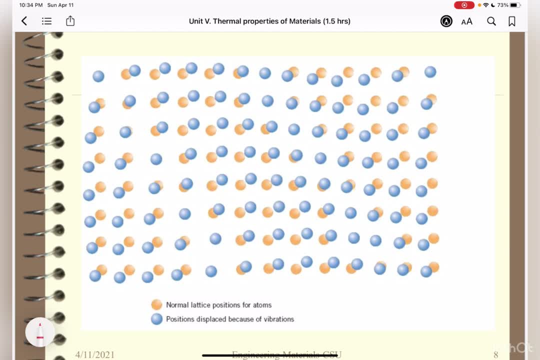 balls here and then the blue balls would give you the positions displaced because of vibration. you would know that these vibrations are coordinated in such a way that the traveling lattice waves are produced. So take a look at this one, So you would see wave-like positions. 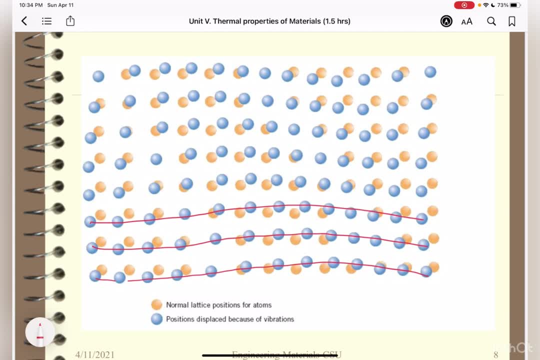 So note that vibrations of adjacent atoms are coupled by virtue of the atomic bonding. So the vibrational thermal energy of a material Consists of a series of these elastic waves which, as all waves, have a range of distribution and frequencies. You've learned that in chemistry or physics. 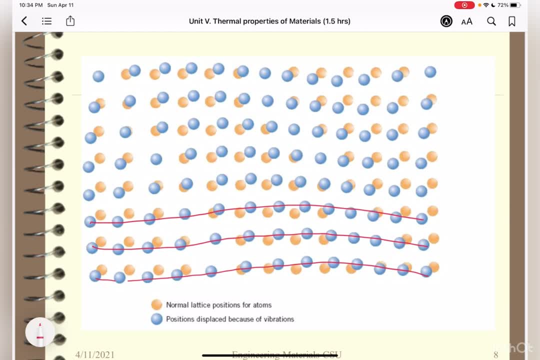 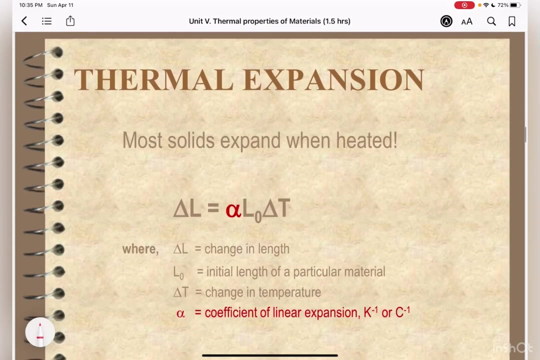 So a single quantum of vibrational energy is what we call as your phonon, And this is analogous to quantum electronic radiation called the photon. Phonon is for vibrational energy And photon is for electromagnetic radiation. Okay, So if we are to deal with thermal expansion, 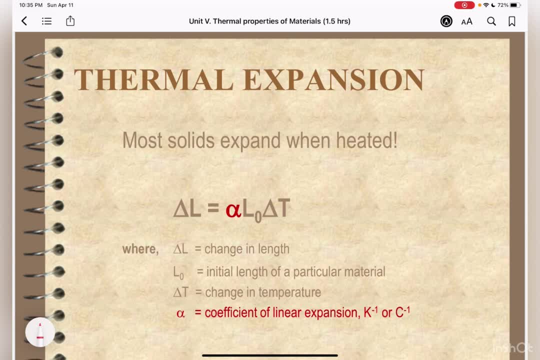 most solid materials expand upon heating and contract when cooled. Let's see the the usual phenomena. So the change in length with temperature for solid material may be expressed. So if there's a change in length, that is your final length minus the initial length, all over the initial length. 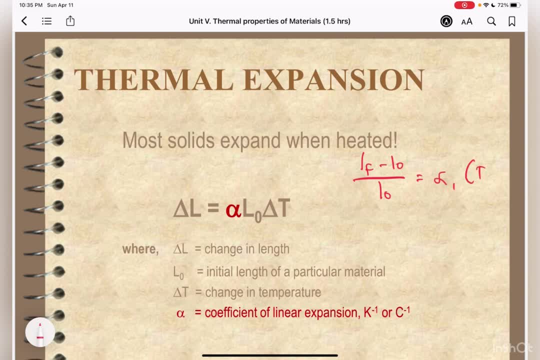 which is equivalent to your alpha one times the temperature final, minus temperature, initial, Or we term this as your delta L. So that's why you have an equation. You have an equation: Delta L is equivalent to alpha L or delta T. Take note that alpha here is the coefficient of thermal of linear expansion. 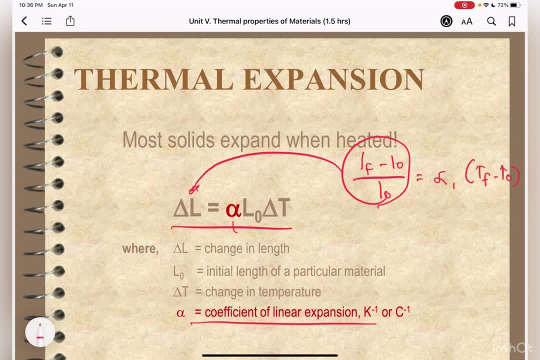 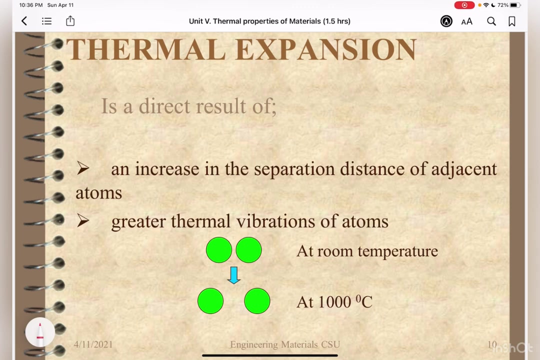 which is it's a material property that is indicative of the extent to which a material expands upon heating, And usually its unit is per Kelvin or per Celsius degree degree. You have to remember that. Okay, So we talk about thermal expansion. It is actually a direct result of an increase in the separation distance of the adjacent atoms. 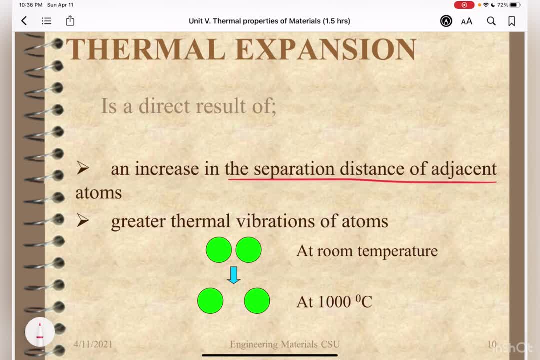 And of course we know that the greater thermal vibration of atoms, say, for example, at room temperature. this is the position of the atoms Now, if we hit that one, there would be vibrational energy, And that you have a farther distance between two molecules at 1000 degrees Celsius. 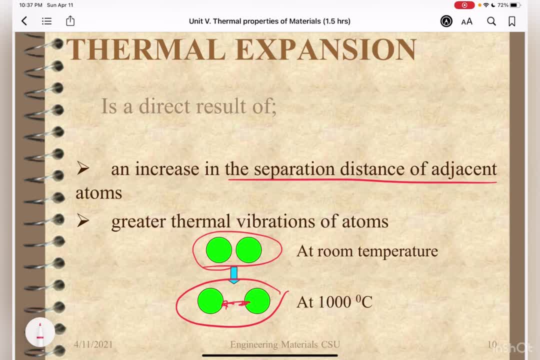 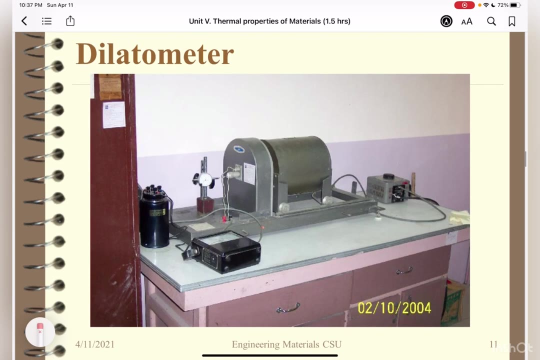 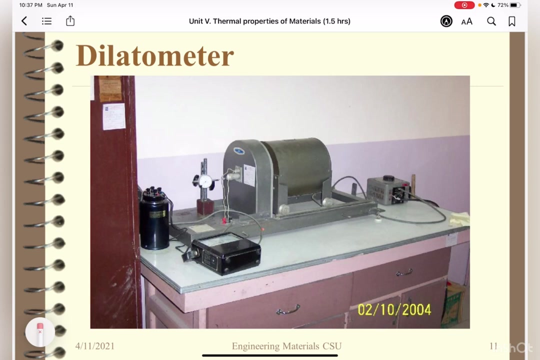 So it's a separation distance. Okay, So, from an atomic perspective, this thermal expansion is reflected by an increase in the average distance between atoms. Okay, So I have here a dilatometer which is found in found at the DOST material science division. 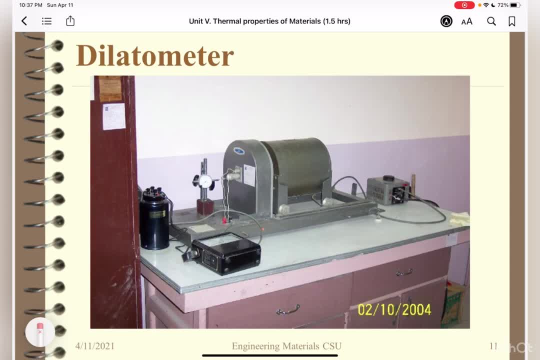 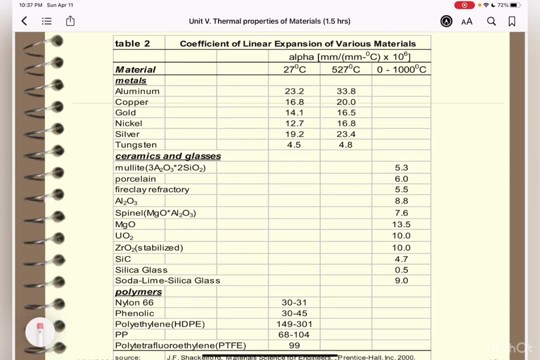 So it's used to measure thermal expansion. So I think I have here the coefficient of linear expansion of various materials. And for each class of materials- either metals, metals, ceramics or polymers- the greater the atomic binding energy, the lower the coefficient of linear expansion. 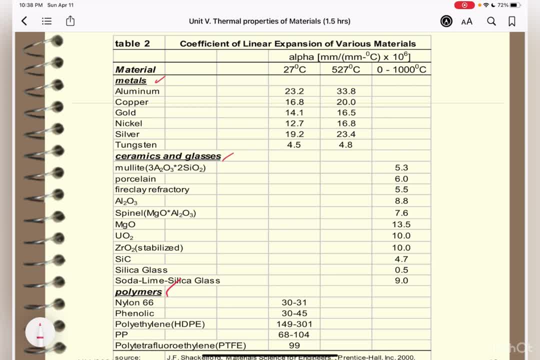 So check the values of ceramics, which has relatively strong interatomic bonding forces, So, as expected, they have low coefficient of thermal expansion. The highest alpha values are found in linear and branched polymers. Okay, So the because of the 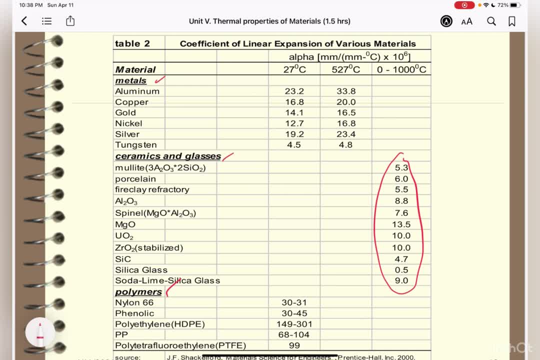 because of the secondary intermolecular bonds are weak and there is a minimum minimum of cross-linking. So if polymers are covalently bound, expect for low alpha values, Say, for example, the phenolic resins. Okay. 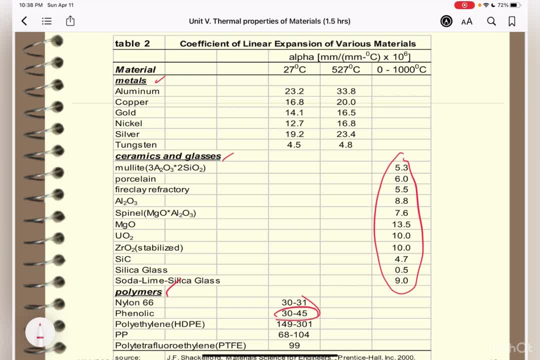 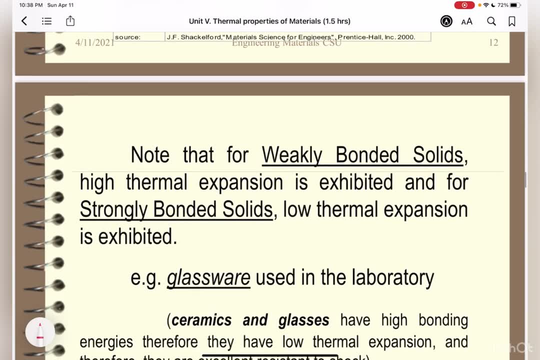 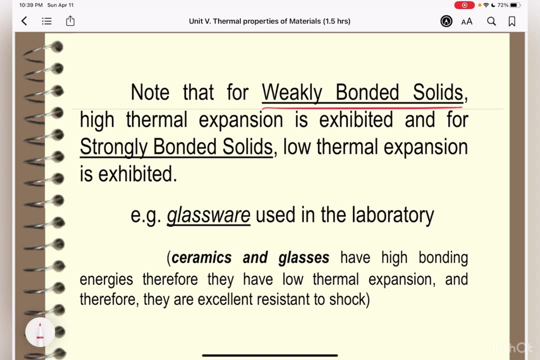 So for metals they have values that are intermediate between your ceramics and your polymers, So they're in between. Okay, So you have to note that weakly bonded solids, high thermal expansion is exhibited and for strongly bonded solids, low thermal expansion. 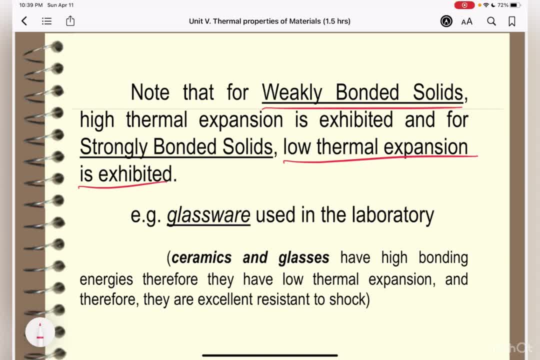 I think I have included this in some of the quizzes that I've done before. So one good example is why glassware is used in the laboratory: because ceramics and glasses have high bonding energies. Therefore they have low thermal expansion and they are excellent resistance to. 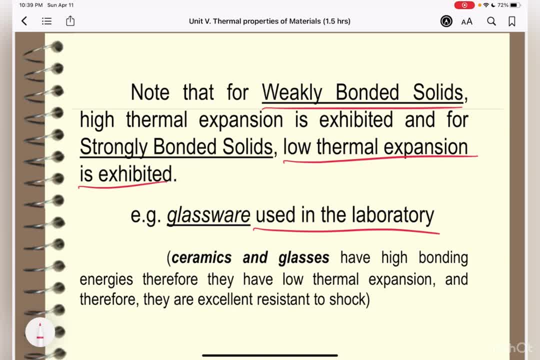 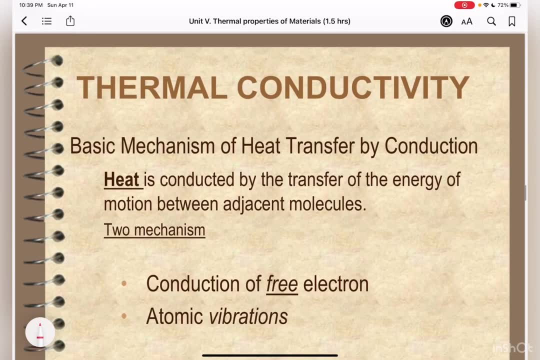 resistant to shock. That's why parents or your mother who have Pyrex, you can use Pyrex glass straight from the oven and to the dining table. Okay, Okay, Let's define what thermal conductivity is. So the basic mechanism of heat transfer by conduction. 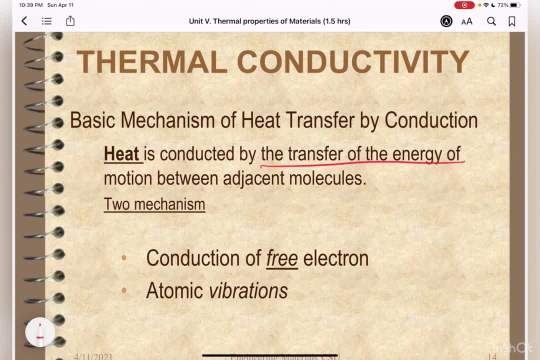 heat is conducted by the transfer of energy, of motion, between adjacent molecules, And there are two mechanisms to do that. One is conduction of heat by free electron, and what we've discussed a while back is due to atomic vibration, So the transport of thermal energy. 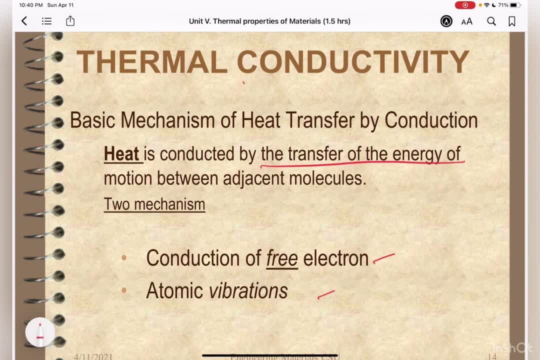 from high to low temperature regions of a material is termed your thermal conduction, So it's always from high region to low temperature region. So for solid materials, heat is transported by the free electrons and by the vibrational lattice waves, or we term that as. 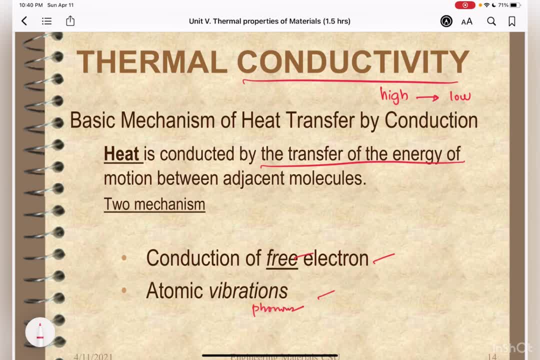 phonons. Okay. So the high thermal conductivities for relatively pure metals are due to the large number of free electrons and also the efficiency with which these electrons transport thermal energy. And, by contrast, of course, ceramics and polymers are poor thermal conductors. 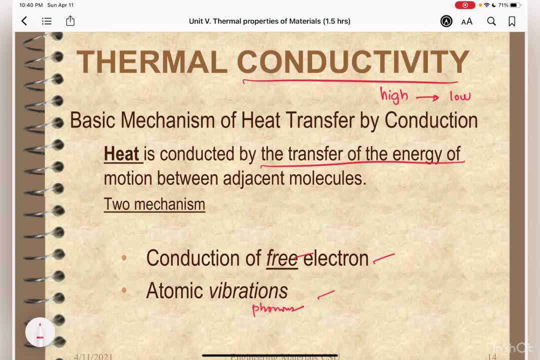 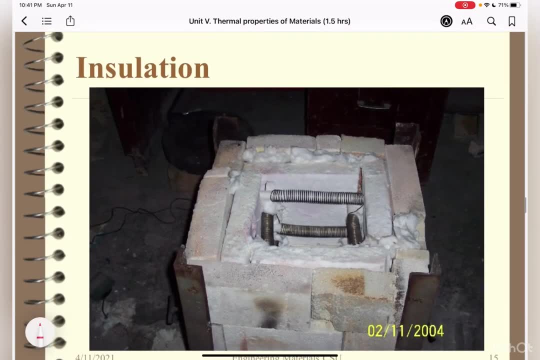 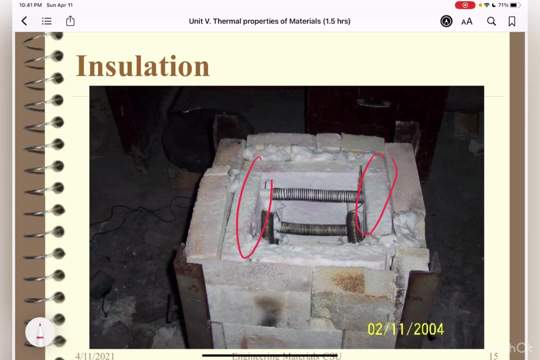 because free electron concentration are low And that phonon conduction predominates. Okay, As you can see in this figure, I have here thermal insulators. This is your ceramics, Because they have poor thermal conductivity, like we term this as non-metallic ceramics. 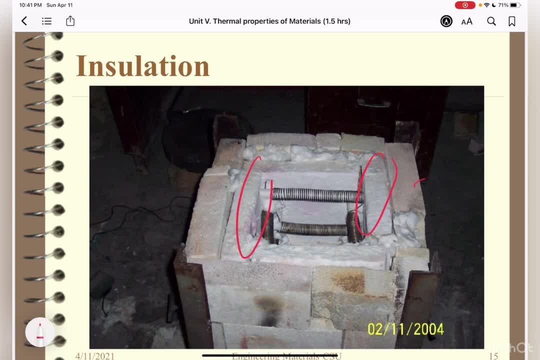 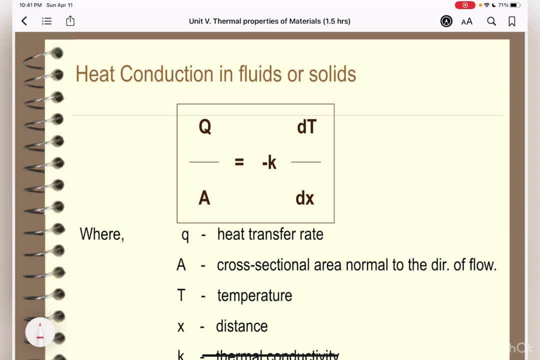 or the bricks. They lack large numbers of free electrons. Okay, Let's discuss more about heat conduction. So heat conduction in free electrons, fluids or solids given by this equation- This is actually the popular Fourier equation. You will be dealing most of this. 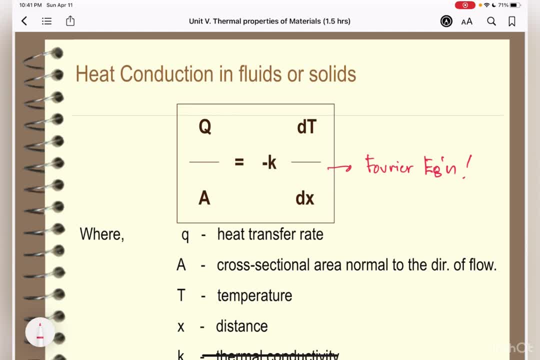 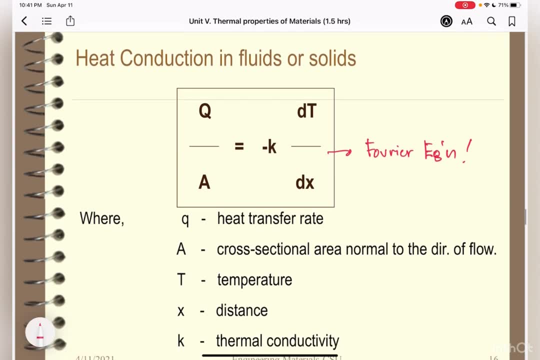 when you take up heat and mass transfer, I think by next semester and hopefully I'll still be your professor in the subject. So from this equation your Q is a heat transfer Weight. A is a cross-sectional area normal to the direction of flow. 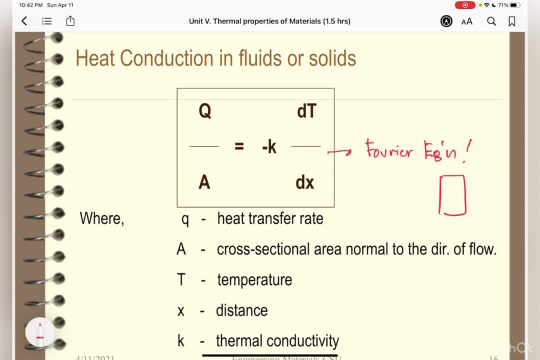 So if you say assuming, if you have here a cube, So the area perpendicular or normal to the direction of the heat flow is just this area here, This area of this, the heat flow. Okay, So Q is of course the temperature, X is the distance. 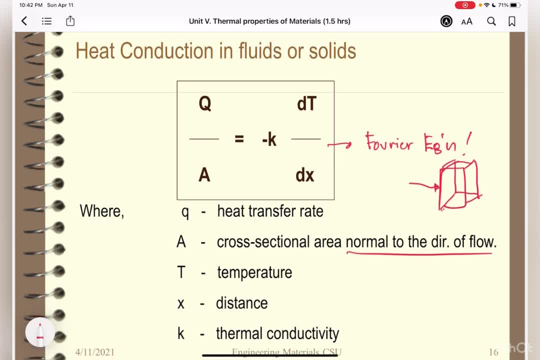 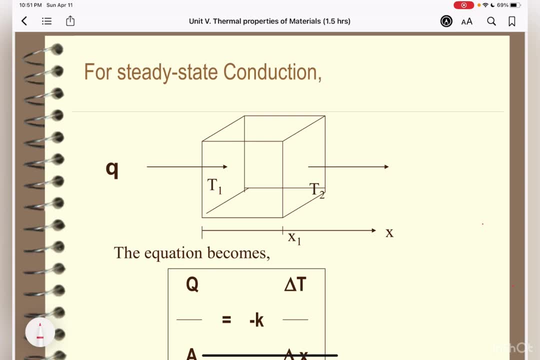 and K is the thermal conductivity of the material being under study. Okay, So let's consider for a steady-state conduction. When we say steady-state conduction, the heat flow is constant with time. So here, heat flow is constant with time. 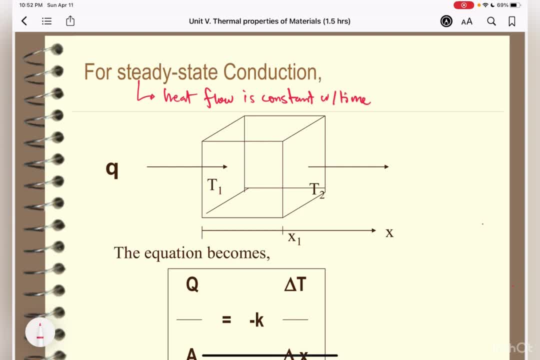 So how is that? So, assuming say, for example, we have a time 1 pm, The change in temperature is from 100 degrees to 40 degrees centigrade. After one hour time 2 pm, still the change in temperature. 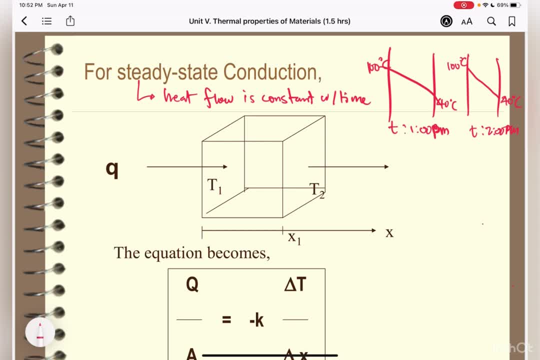 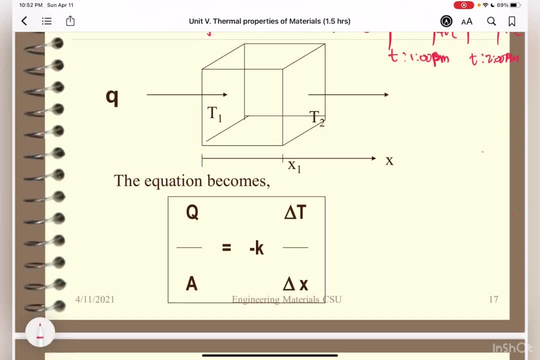 or delta T would still be 60 degrees. So that's a steady-state heat conduction. So I'd like to derive the equation for Fourier, which is actually given by this equation: Q over A equals negative K, delta T over delta X. 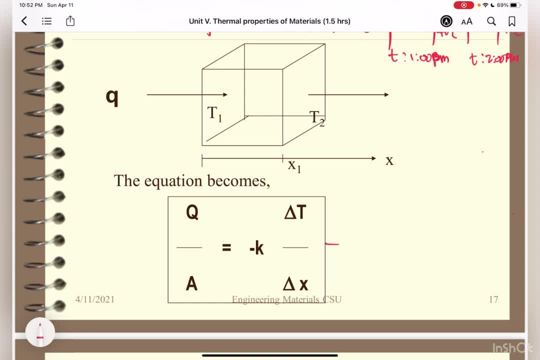 So later, when you take your hemat or your heat and mass transfer, you'll be learning more about the molecular transport equations, three equations: your molecular transport of mass, which is with your deals, with your diffusion, etc. Or the famous equation for the molecular transport of mass. 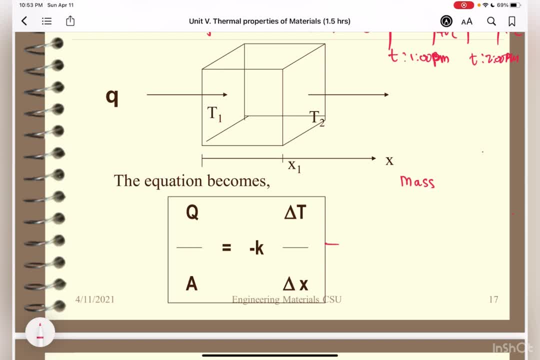 is actually your fixed equation. I don't know if you've encountered this already. Second is your molecular transport of momentum in your fluid flow, And this is your Newton's equation, And our focus for now is the molecular transport of heat, or the Fourier equation. 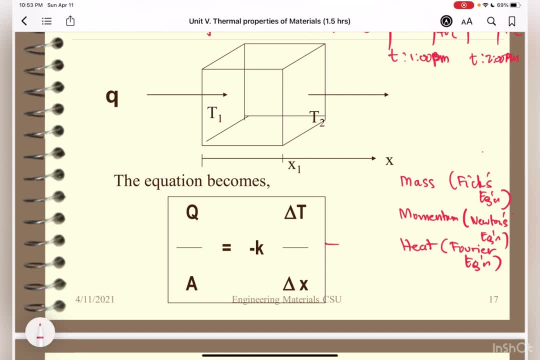 Although in your heat and mass transfer there are different types of molecular transport of heat. It can either be conduction, convection, radiation, evaporation, etc. Okay, What's the basis of these three equations? The basis of this actually is: 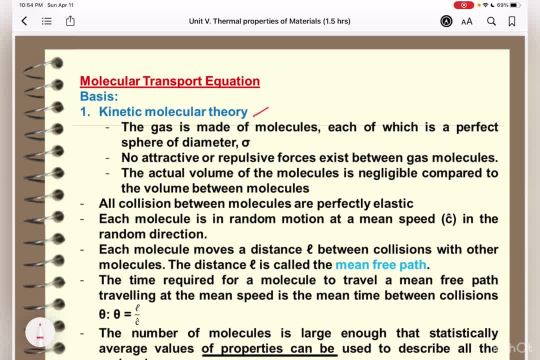 the first is, you have the kinetic molecular theory. What's in the kinetic molecular theory, Chemistry 1 or Chemistry 2?? First is the gases made of molecules, each of which is perfect, which has a perfect diameter of, say, this one. 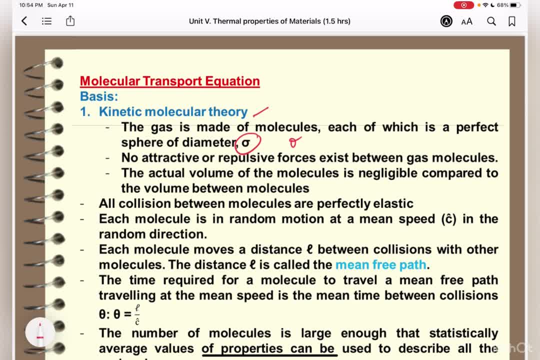 So no attractive or repulsive forces exist between molecules. That's why say: this is molecule 1,, it bumps with molecule 2, since they're perfectly elastic, Even if they bump with each other they would have no attractive or repulsive forces. 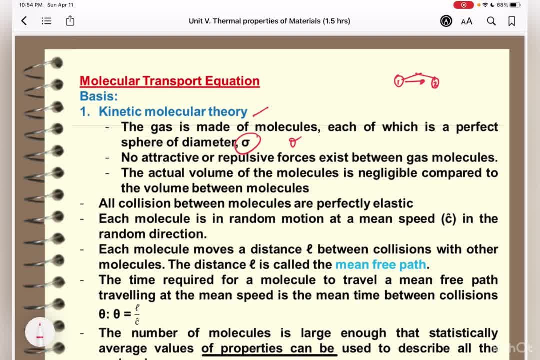 Okay, So the actual volume of the molecules is negligible compared to the volume between molecules. So it's: the total volume is so large compared to the volume of each of the molecule. I've said a while back, all collision between molecules are perfectly elastic. 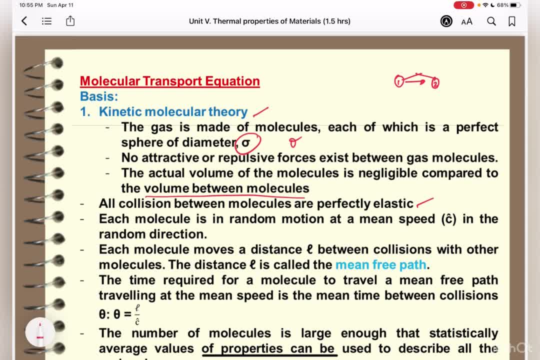 So if it is perfectly elastic they don't bend each other Once they bump they could just freely distance from each other. So each molecule is in a random motion at the mean speed of c-bar in the random direction. So if I have this molecule, 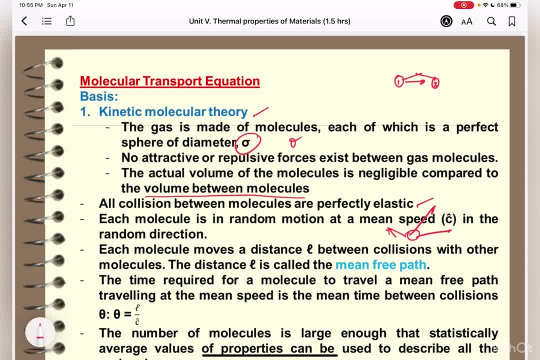 it can travel freely to any direction with a speed of c-bar. Now each molecule moves a distance l between collisions with other molecules. So say for example earlier, if this molecule collides with molecule 2, the total distance it traveled is given by l. 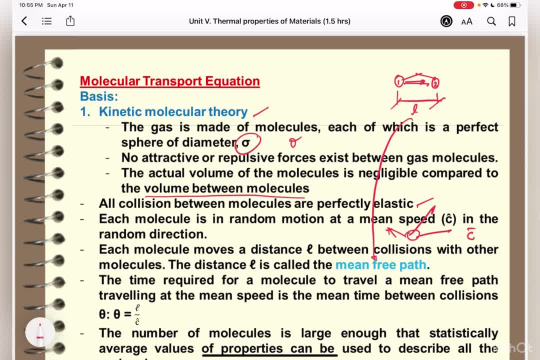 And we term this as your mean free path. Now, the time required for a molecule to travel a mean free path, traveling at a mean speed, c-bar is a mean time between collisions, or theta is equal to your l over c-bar. 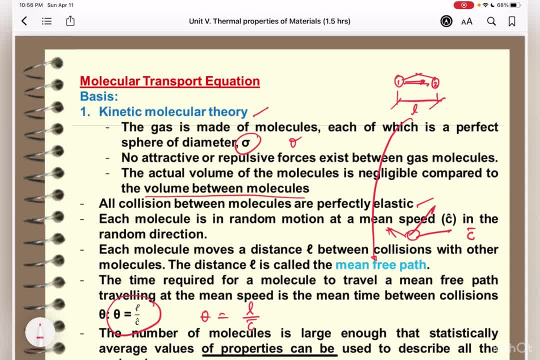 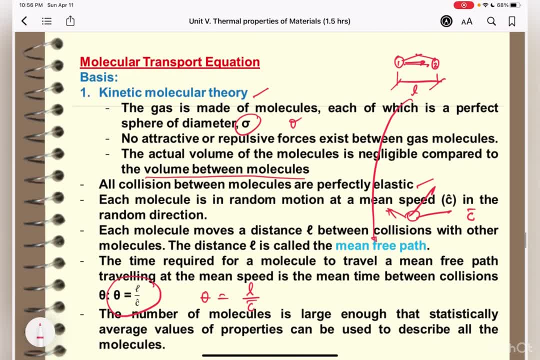 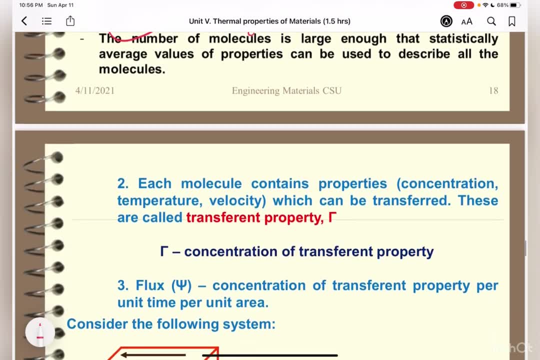 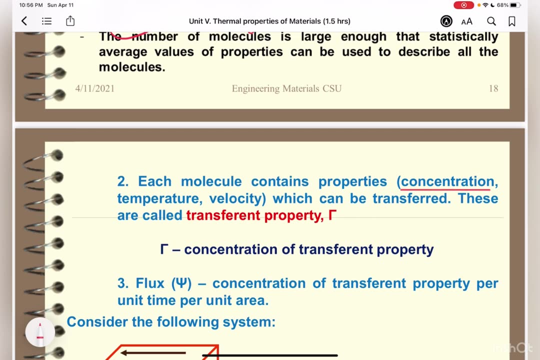 And the number of molecules is large enough that statistically average values of properties can be used to describe all the molecules. Okay, So you've learned that from your kinetic molecular theory. The second basis is that each molecule contains properties, either concentration, so that's for your molecular transport of mass. 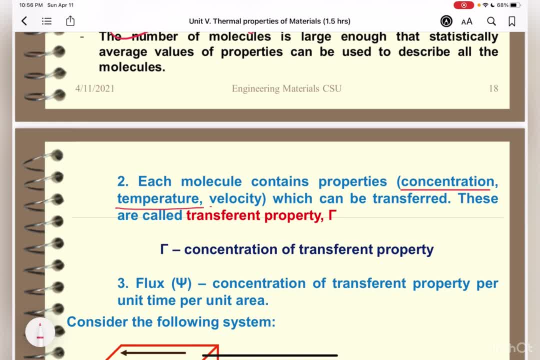 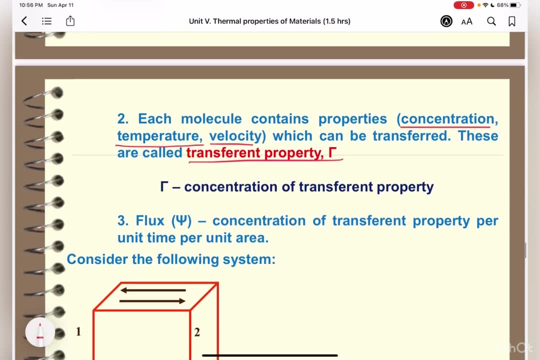 a temperature, or your molecular transport of heat or velocity, that's, your molecular transport of momentum which can be transferred, And these are called your transparent property or your gamma. So we term gamma as a concentration of your transparent property. And the last basis. 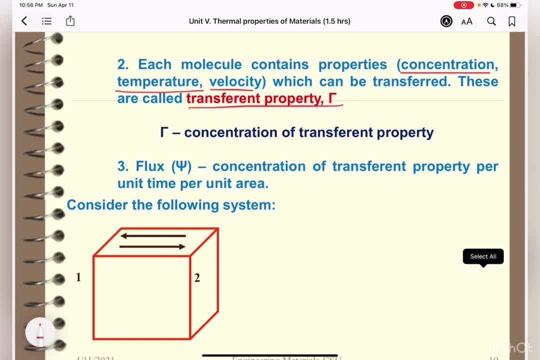 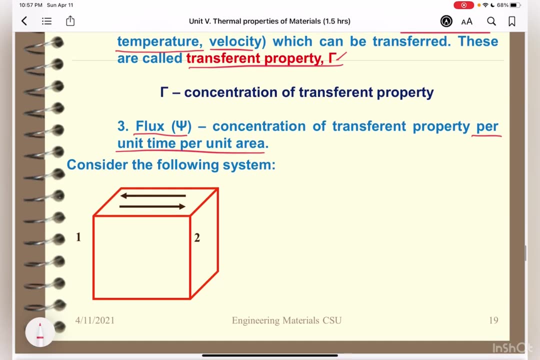 for this molecular transport equation is that there must be a flux, which is a concentration of the transparent property per unit time, per unit area. Okay, Let's consider this following system, Assuming I have here molecules traveling from. Let's see if I got. 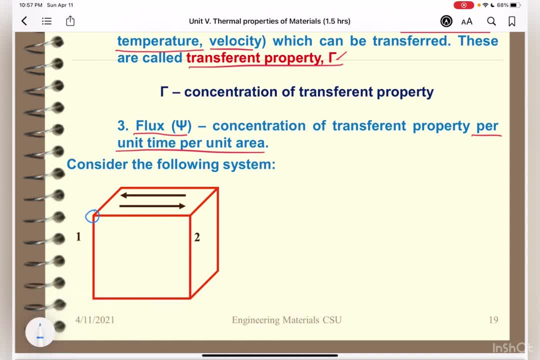 Let's see. So you may have molecule one And then these are some of the different molecules. Okay, So the concentration of molecule one moving from this plane one to plane two. so at the end, moving from plane one to plane two. 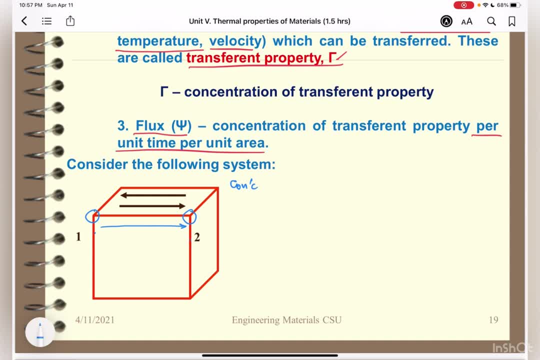 therefore, the concentration of that- Okay, let's try The concentration of molecule moving from plane one to plane two- would be the transparent property, or the concentration, or that's gamma over six. Why six? Because this molecule can travel. 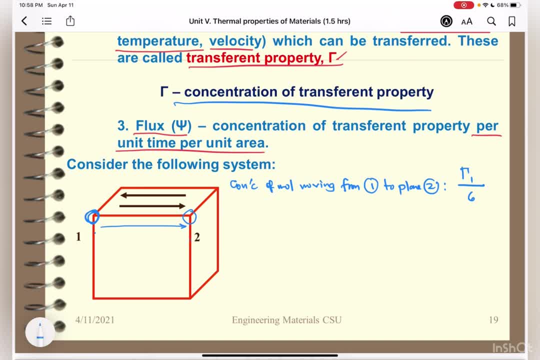 say in the back. let's say, assuming that this is a cube, it can travel six different on the six different planes. It can either be on top right side, assuming that's heavier, Okay, Top, bottom, right side, left side. 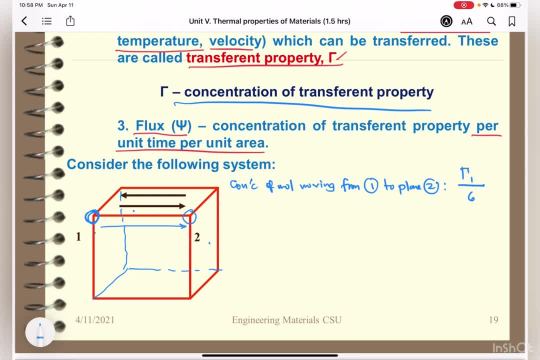 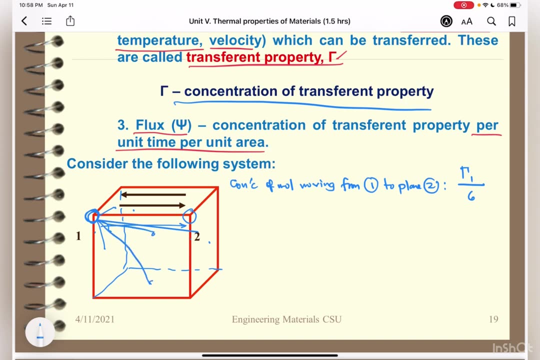 and then the front and the back. So that's actually six. So it can travel, can bump the top, it can bump the front, the right side, the left side, the bottom and the back and front. So you have six phases. 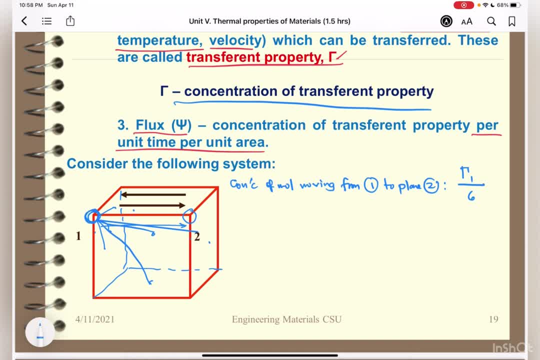 that this molecule could actually travel. Okay, Therefore, the flux, Therefore the flux of the molecule moving from plane one to plane two, would be given by gamma one, or there's a transparent property divided by six times, of course. 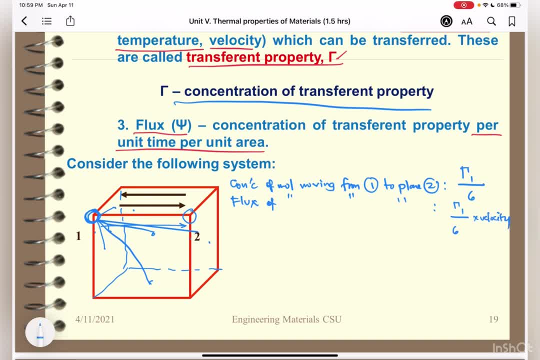 the velocity, Okay, Or this could be gamma, one over six times your C bar, or the speed, But we said earlier, C bar could also be L or theta is L over C bar. right, You have, theta is L over C bar. 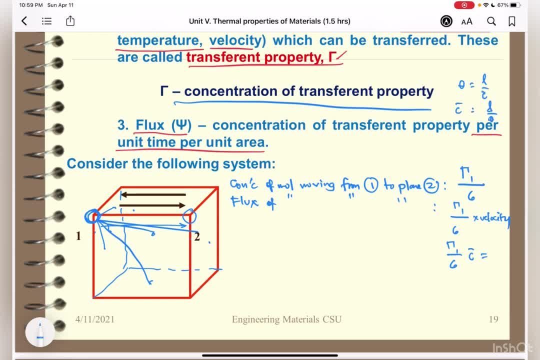 Therefore C bar could be L over theta, Or that would be gamma one over six times L over theta Times. this is L over theta. So that's the flux of the molecule moving from plane one to plane two. Now let's consider 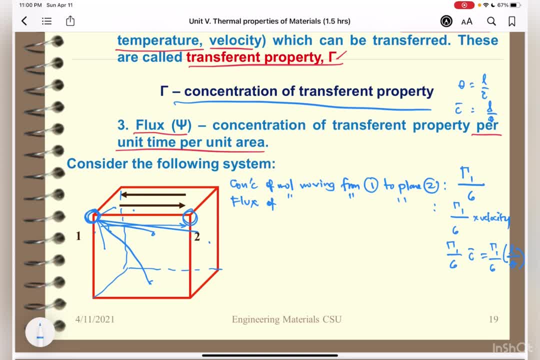 going back, if it is the flux, the concentration, the concentration of of molecule moving from plane two to plane one, That could be gamma, distilled gamma, two over six, And the flux would definitely be. what's the flux? It could be? 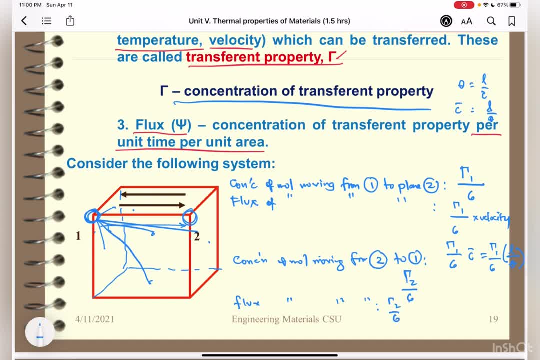 your gamma two over six. Take note: this is negative L over theta because it's going on the left direction, Assuming that going to the right or forward moving would just be positive. Therefore, this is a negative distance. Okay Now. 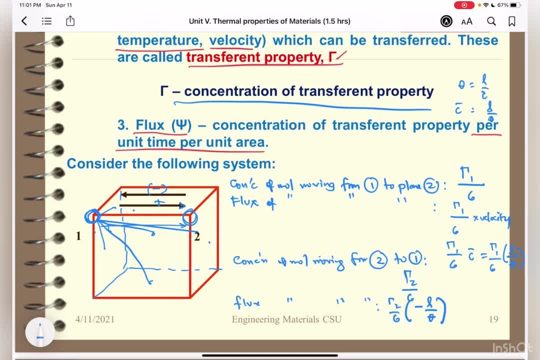 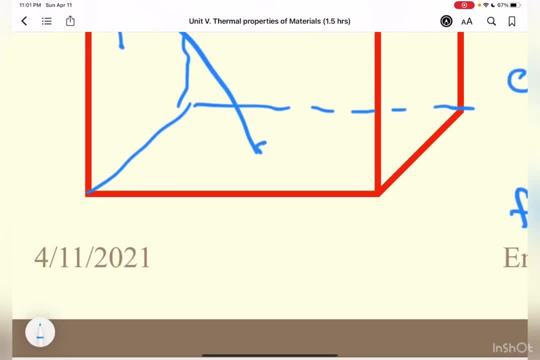 if we are to consider the net change of flux from one to two. so net change of flux from one to two, this could be gamma one over six times L over theta, plus your gamma two over six. This time it's negative L over theta. 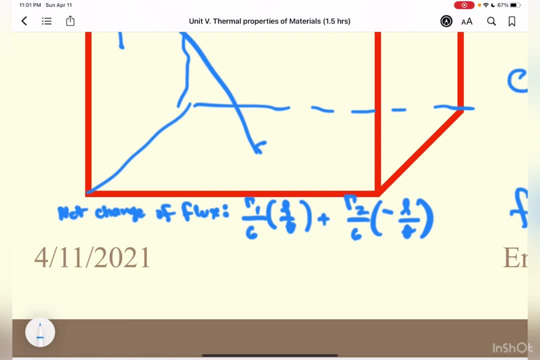 Or we could say that this could be negative L over six theta times gamma two minus gamma one, Right So negative L over six theta gamma two minus gamma one, Or we term this gamma two over gamma one to be the change in the 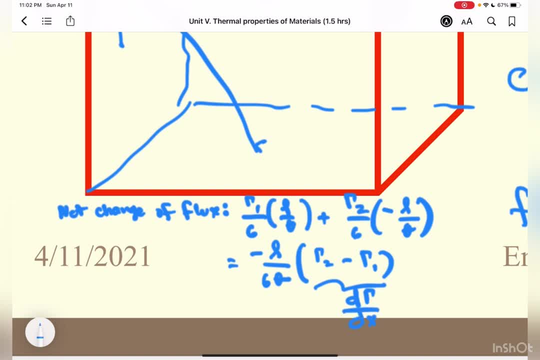 transferent property over dx. Okay Times L If I'm to substitute negative L. therefore, all over, what is six theta? Theta is L over C, L over C. This is six times derivative of gamma over dx, times L. 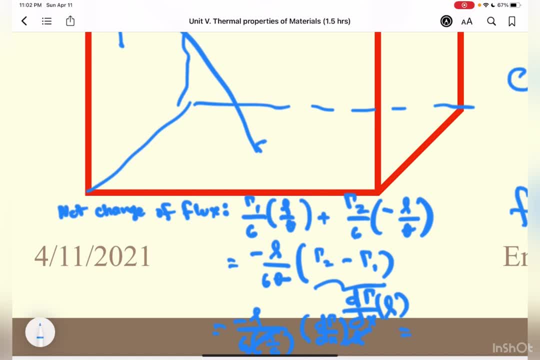 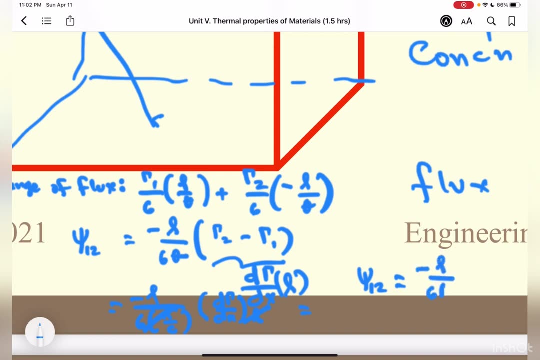 Or this cancels out with the L there. Finally, I would have the equation flux from one to two, Or assuming this flux one to two, therefore, would be equivalent to negative L over six theta Wrong. Sorry for that. 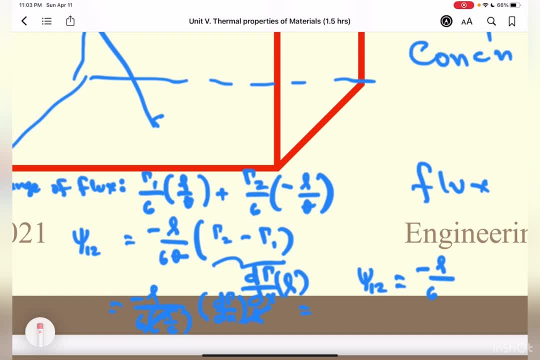 It's not six theta, but it is six over C, Or I could bring C here: Negative L C over six, negative L C over six, negative L C over six. derivative of your transferent property, gamma over dx, And this is what we call. 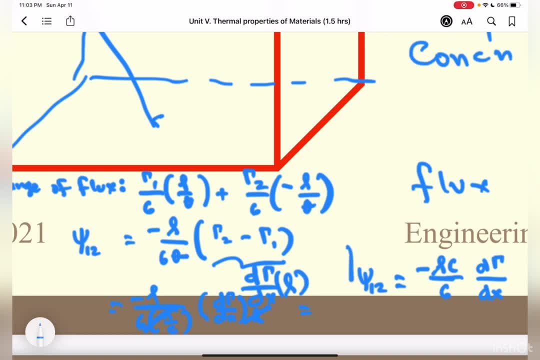 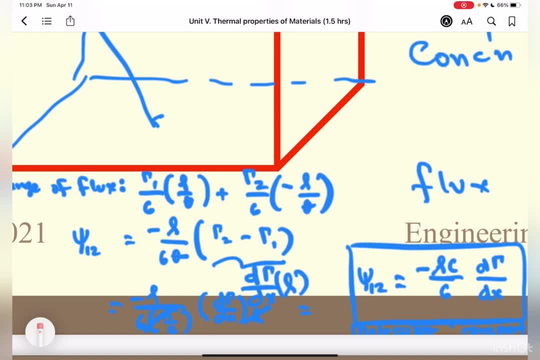 that's your flux is equivalent to negative L C bar. sorry, L C bar over six derivative of gamma over dx. Okay, Okay, So this is actually your molecular transferent property of mass transport equation. So, the mass transport equation, the heat. 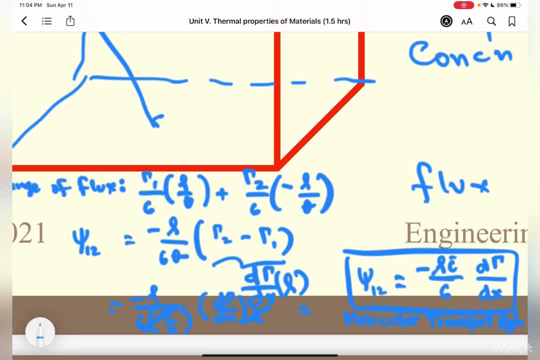 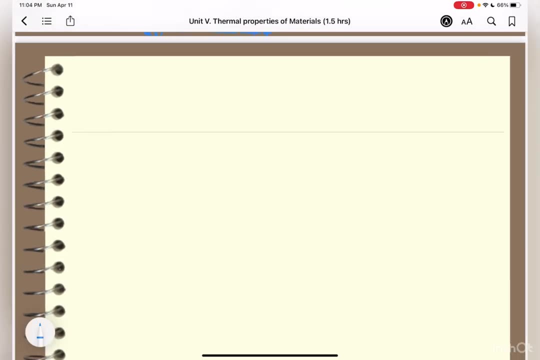 transport equation and your momentum transport equation would have this as its general equation. Okay, Let's proceed with your heat transport equation, or the derivation of your heat transport equation. The Fourier recall: flux is equivalent to negative L, C bar over six derivative of the. 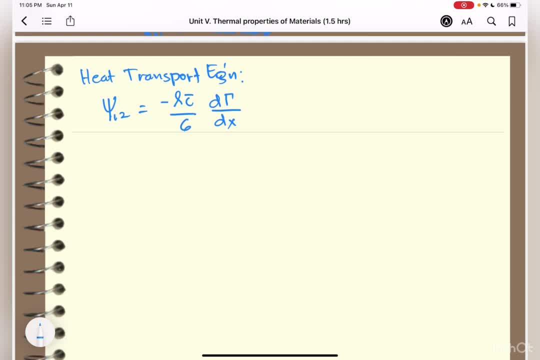 transferent property over dx. Okay, So this is your molecular transport equation. The first is: there should be. what's the requirement? Temperature difference should exist, Otherwise full energy transport. Okay, So temperature difference should exist. Second: 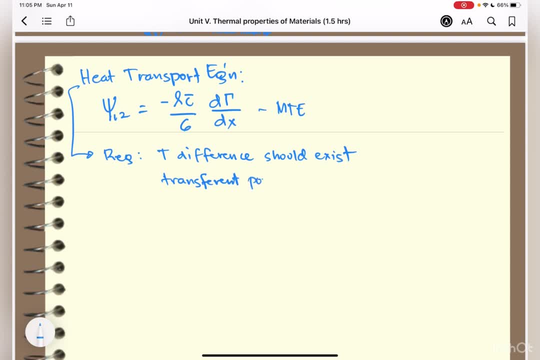 what is our transferent property Gamma? There should be concentration of thermal energy, Or what is that concentration? My CA would therefore be rho CP T, But temperature is your derivative of your transferent property. So if your transferent 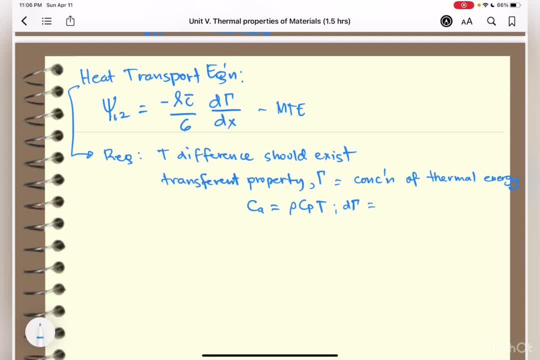 property is your CA? derivative of your gamma or derivative of the transferent property would be equivalent to rho, CP, T. Take note, your rho and CP are, of course, your constant. Okay, The third is your heat transfer per unit area. 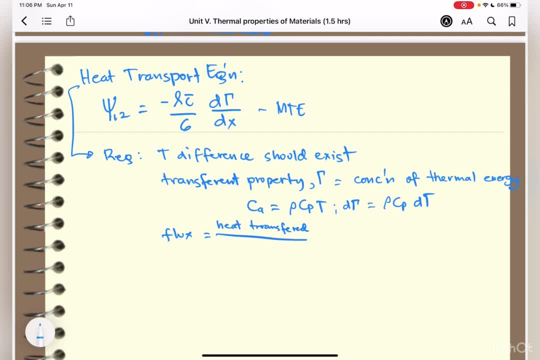 Heat transfer, of course, is the heat transfer per unit time In flux. it should be the transferent property per unit time, per unit area. So we term that as your Q over A. Okay, Now let's plug this transferent. 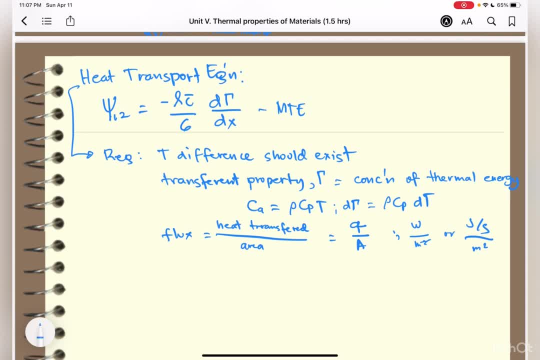 property flux to our MTE. So flux is equivalent to what is our flux. Your Q over A is equivalent to negative LC bar over 6 times the derivative of your transferent property rho Cp dt over dx. Take note that this. 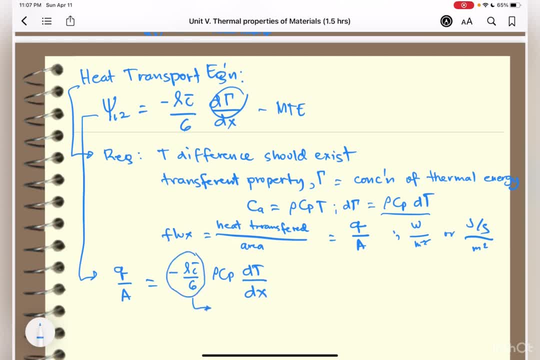 LC bar here. negative LC bar is what we call as your alpha, or it is your thermal diffusivity In the property of materials. in your handbook you can find this one. If that is alpha, I would have my flux Q over. 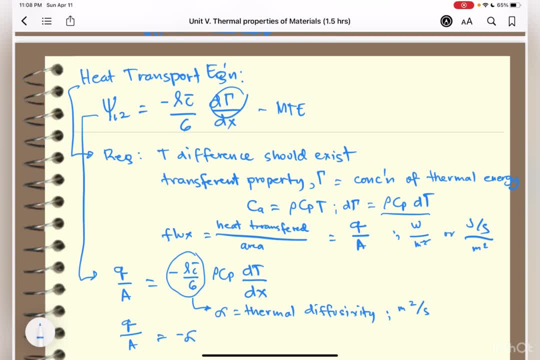 A is equivalent to negative alpha rho Cp: dt over dx. And what is this constant here? Your alpha rho Cp is what we call thermal conductivity. This is your flux, Q over A, which is term K. Therefore, I would arrive at an equation that is: 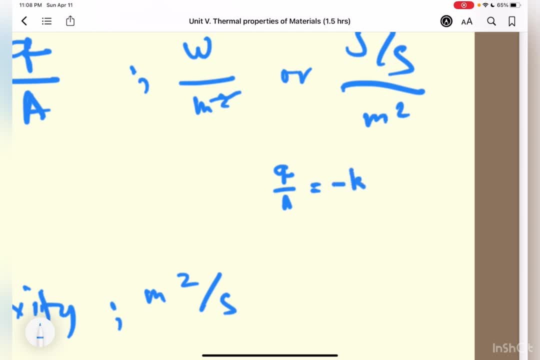 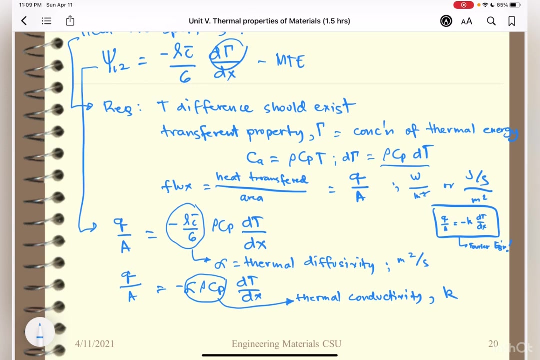 my flux Q over A is equivalent to negative K, which is your rho Cp alpha dt over dx. So this is my flux Q over A. Now I have an understanding how the Fourier equation was derived. Wait for your hematra. I won't. 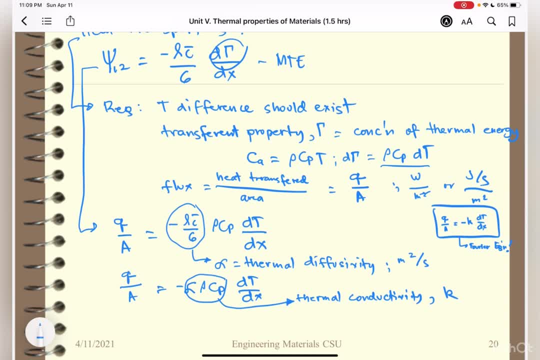 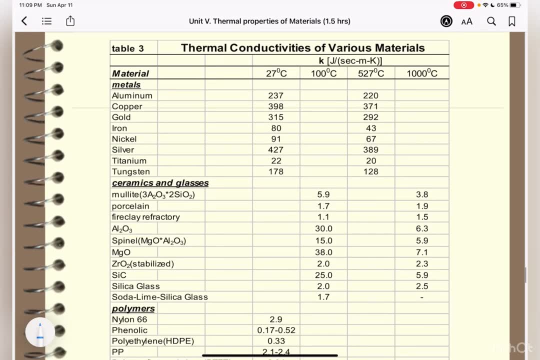 be discussing now your molecular transport of heat mass and your molecular transport of heat mass. So this is my flux Q over A. So this is my flux Q over A. This is my flux Q over A. So this is my flux. 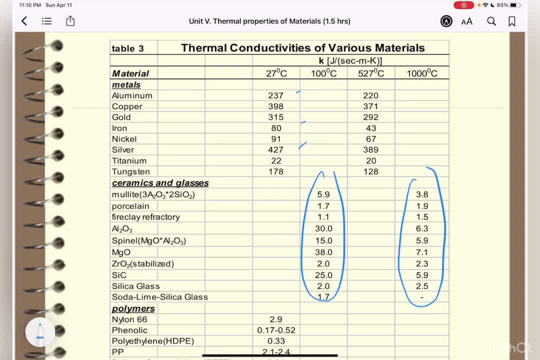 Q over A. So this is my flux Q over B. I would like to ask for this because this is my flux Q over A. So let's write this formula: This is my flux Q over A. So this is my. 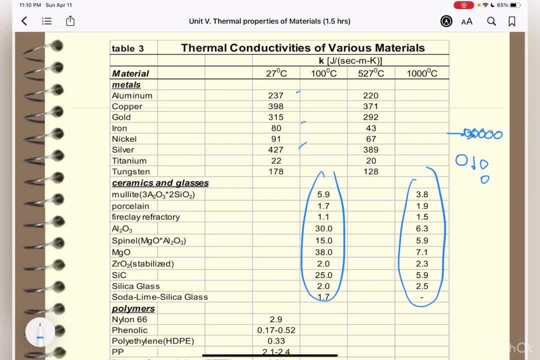 flux Q over A. So if I use this mass here harder or you need more energy, that's why you have a low thermal conductivity. so this internal pores usually contain still air and air has a very low thermal conductivity. so if these are spaces or air, air would have thermal conductivity of just around- imagine 0.02 watt per meter. 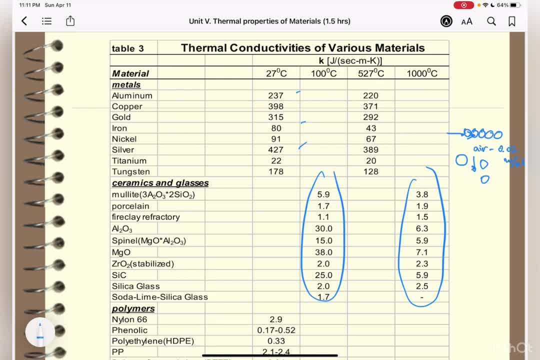 Kelvin. so heat transfer across these pores that contain still air is ordinarily slow and inefficient. now also, polymers are often utilized as thermal insulators because of their- if you have, of course, a very low thermal conductivity. you're not a good conductor, therefore you are a good insulator. so, as with ceramics, their insulative properties may be further. 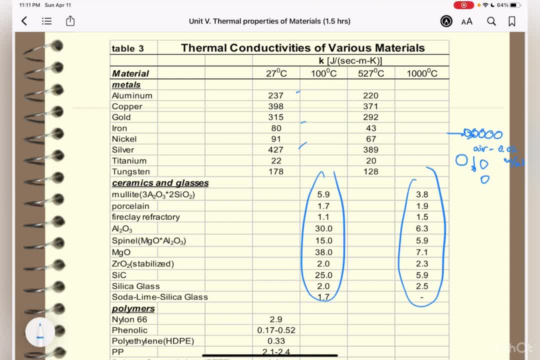 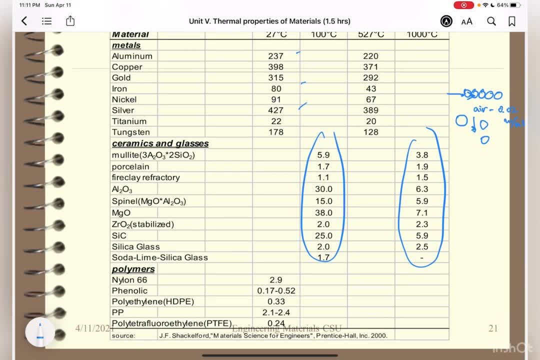 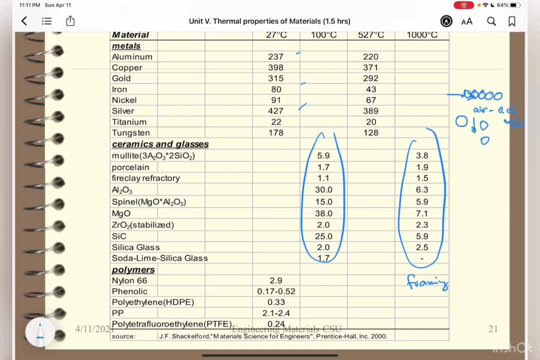 enhanced by the use of thermal insulators, by the introduction of small pores, which are ordinarily introduced by foaming- so some polymers- or with ceramics foaming during polymerization. that's why our most commonly used for drinking cups, your coffee cups at your favorite fast-food joints, and insulating chest are foam polystyrene. 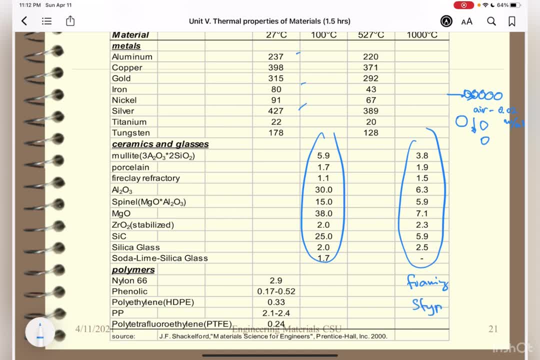 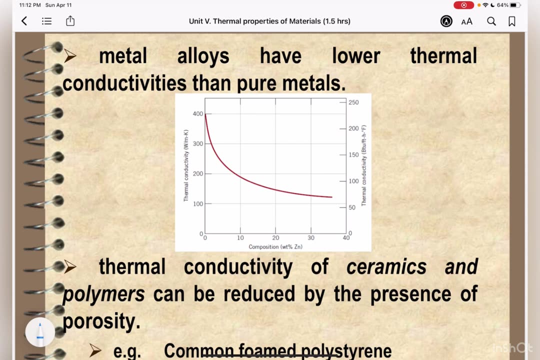 or we call that as your foam, polystyrene, as your styrofoam. it's some styrofoam, because it is being formed during polymerization. okay, so we have here metal. I always, always also have lower thermal conductivities than pure metals. why is? 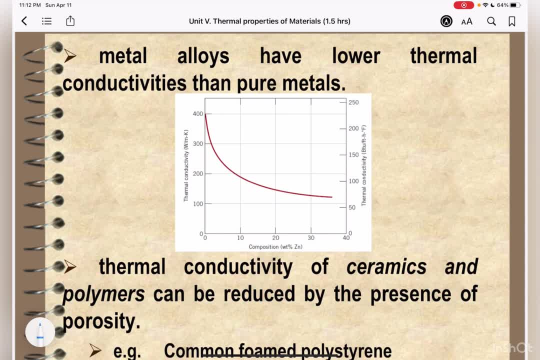 that because alloying metals with impurities result in reduction in the thermal conductivity for the same reason that the electrical conductivity is also diminished. so this is due to the fact that impurity, so alloys would have impurities, so this impurity atom, especially if it is in solid solution, act as a scattering center, so lowering the efficiency of electron motion. so 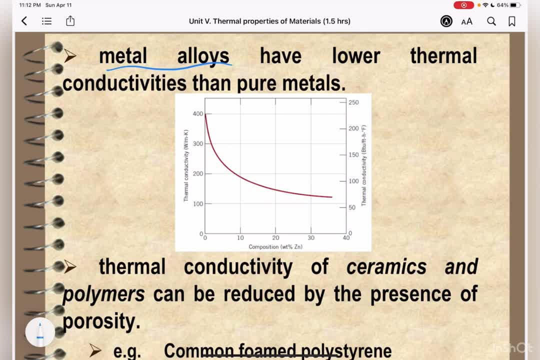 one good example is shown in this figure. you have a plot of thermal conductivity versus composition for a copper zinc alloy. so if you have a copper zinc alloy, you take note that the higher the zinc content, the lower is your thermal conductivity, as shown by this curve here. so if it is pure copper, 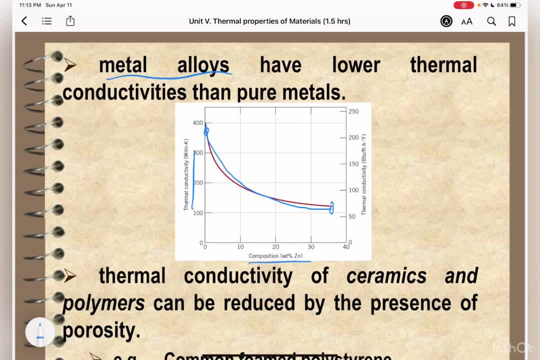 so zero zinc, you have a very high, almost 400 watt per meter kelvin for thermal conductivity. but as you increase- take note, as you increase percentage weight percent of zinc, you have a lower conductivity. so thermal conductivity of ceramics and polymers can be reduced by the presence of, of course, 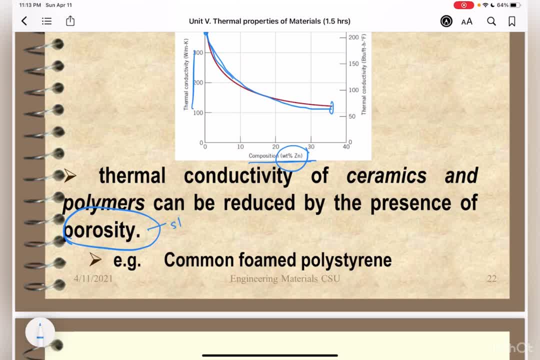 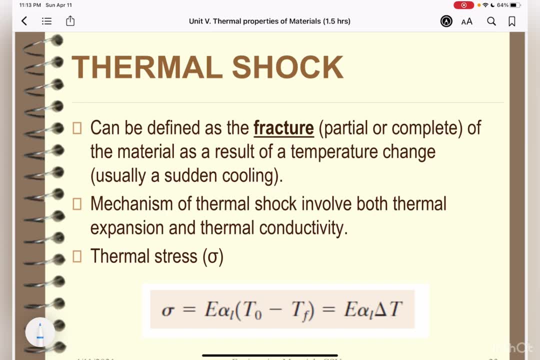 porosity or pores, because it contains still air again. okay, let's define. last one thing about thermal shock. it can be defined as a fracture or partial, partial or complete material as a result of a temperature change, usually, uh, sudden cooling. so this mechanism of thermal shock involves both. 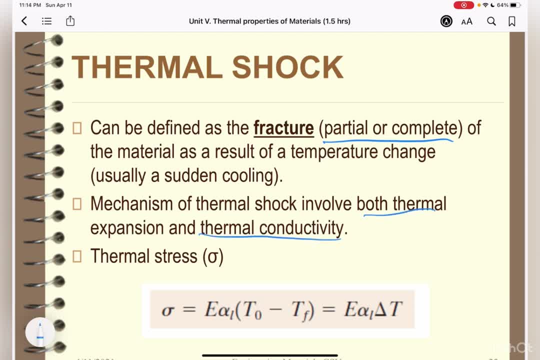 the thermal expansion and thermal conductivity. okay, so thermal stresses. we define what thermal stress? thermal stresses which are introduced in a body as a consequence of thermal changes may lead to fracture or return. that is actually a thermal shock: either uh uh, fracture or undesirable plastic deformation. so the two prime sources of thermal stresses are: 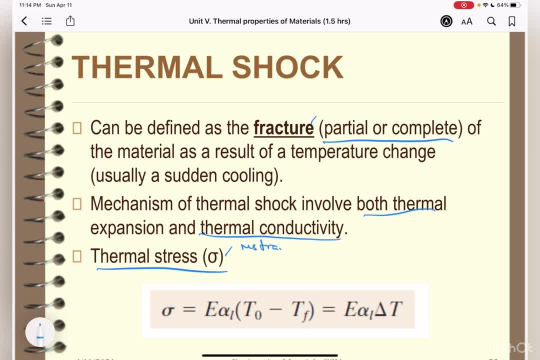 restrained can either be restrained, uh, thermal expansion. when you say restrained thermal expansion, you didn't give time for the material to expand slowly- or a temperature gradient established during heating and cooling. so this one is temperature gradient. it's either sudden cooling or sudden heating. so thermal shock: it is the fracture of a body resulting. 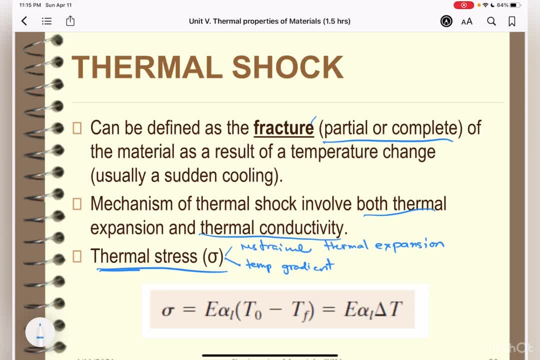 from this thermal stresses. okay. so rapid cooling of brittle bodies more likely to inflate thermal shocks than heating. so the capacity of a material to withstand this kind of failure is we call a thermal shock resistance. so if you are to, if the material could withstand this thermal stresses. 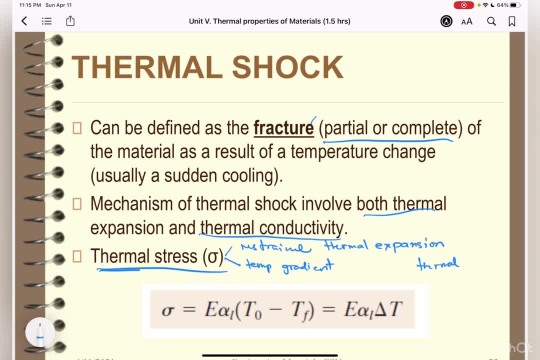 its property would be termed as your thermal shock resistance. okay, this is actually proportional to the fracture strength and the thermal conductivity, and this is inversely proportional to both the modulus of elasticity and coefficient of thermal expansion. that's why we have here that, for thermal stress is equal to E Alpha one initial temperature. 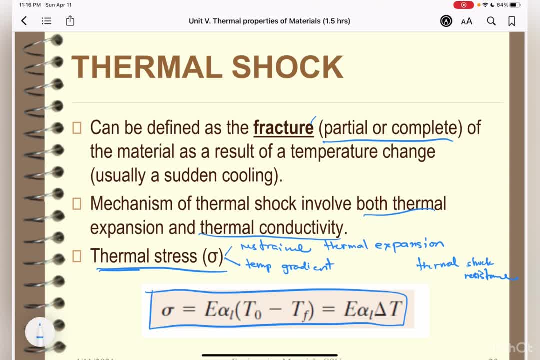 the final temperature, or that's your delta t e. here is what we call in your mechanical properties. this is your modulus of elasticity. alpha is a linear coefficient of thermal expansion and, of course, t o minus t f, for your delta t, is a change in temperature. okay, so upon heating. 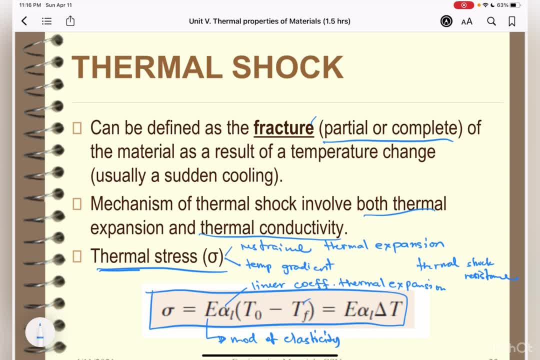 if you hit, of course final temperature is greater than your initial, so t f is greater than t o. what happens if you have t f greater than t o? the stress is uh compressive or your alpha would become, if this is larger than this one, the initial temperature. 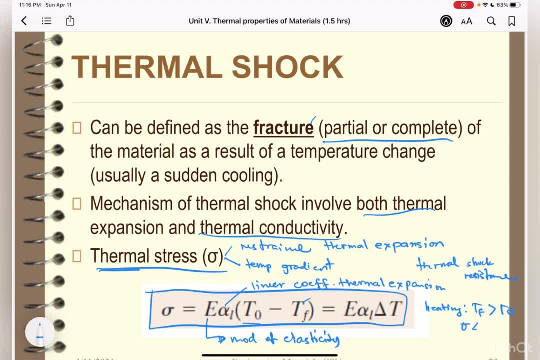 your thermal stress would be less than zero. so you have here say, for example, your rod exponent has been constrained. now if the rod specimen is cooled or your tf is less than your t o, of course you expect that your thermal stress i would be greater than zero. okay, if to is greater than your tf or initial temperature. 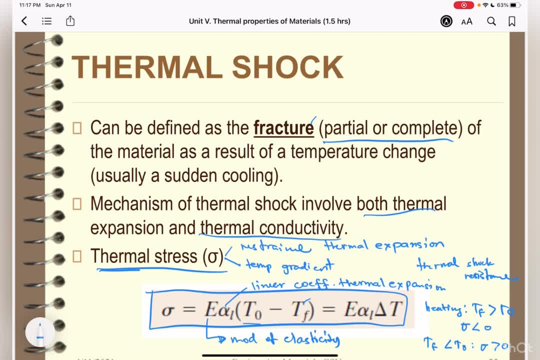 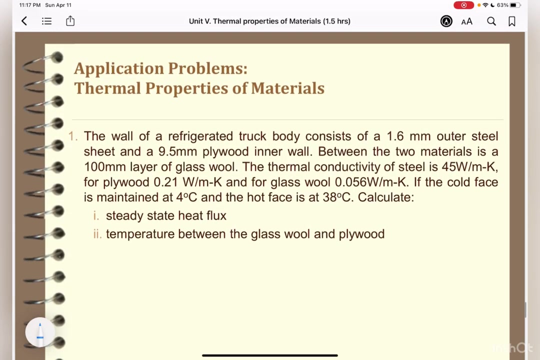 okay, so the stress in this equation is the same as the stress that would be required to elastically compress or elongate the specimen back to its original length after it had been allowed to freely expand or contract with to minus tf as your temperature change. okay, so let's have some simple application problems on thermal properties of materials. 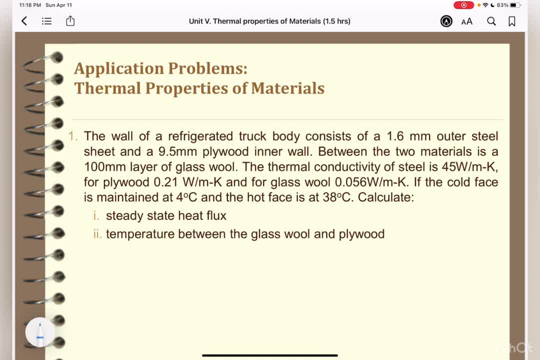 for which, after uh, this i might be, uh, i'll be giving or uploading you some assignments. okay, so let's have number one. the wall of a refrigerated track body consists of a one point point six millimeter outer steel sheet and a nine point five millimeter plywood inner wall between the 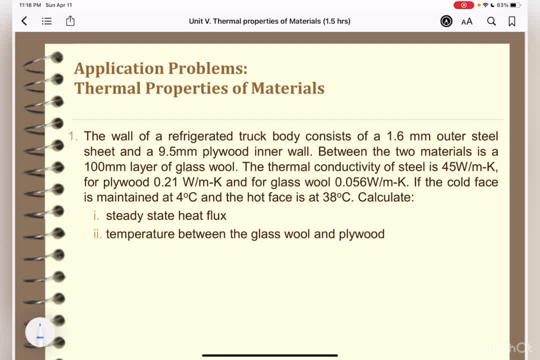 two materials is a hundred millimeter layer of glass wool, so the thermal conductivity of steel is 45 watt per meter kelvin, for plywood is 0.21 and for glass wall is 0.056 watt per meter kelvin if the cold phase is maintained at 4 degrees and the hot phase is at 38 degrees. 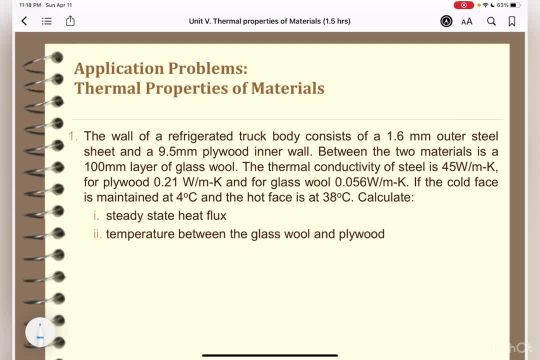 calculate the steady state, heat flow and the temperature between the glass wall and the plywood. okay, so we have here you have, assuming the wall of a refrigerated truck consists of 1.6 millimeter, i have 1.6 mm steel of steel wall and a 9.5 millimeter plywood. between these two materials is 100 mm glass wool. 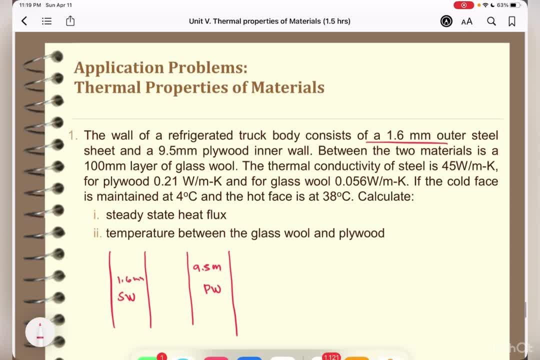 okay, thermal conductivities are given. okay, in steel, 45 watt per meter kelvin. k of your plywood is 15.000 watts per meter kelvin or 0.ентиan watt per meter kelvin of your plywood, and you have a wind resistance. 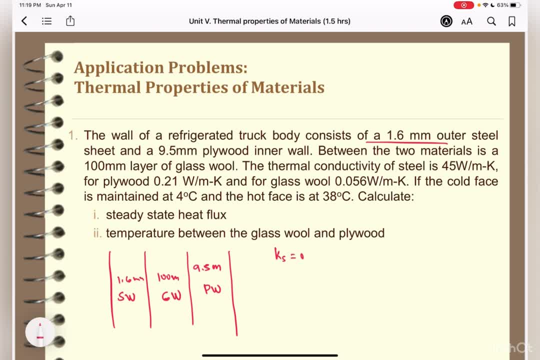 so we have a wide variable of the speed that you want. if you are using a 25 watt per meter Kelvin, you have to have 50 watt per meter Kelvin, which means that the energy Jackie is 0.21 and that of your glass wool is 0.056. 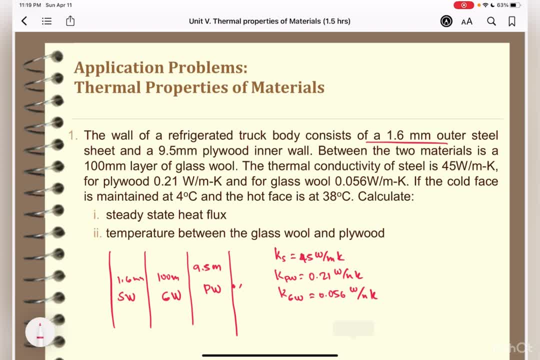 now the cold face is maintained at four degrees- assuming this is four degrees celsius and the outer or the hotter face is at 38 degrees c, we're tasked to get q across this body and the temperature between the glass wool and the plywood, or the temperature at this junction here. 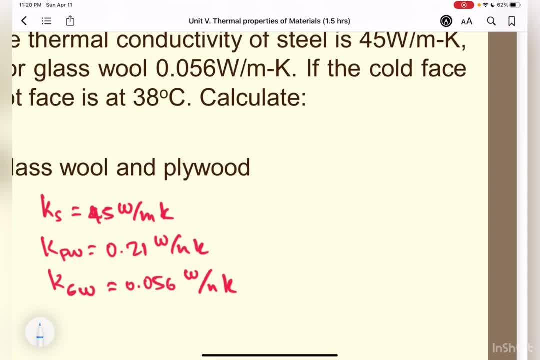 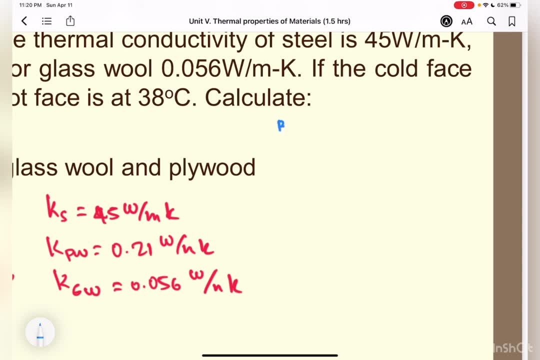 okay, now let's have a basis, say, for example, because we do not know, we do not know the area of the refrigerator trap you have here. the basis is a one meter squared area. know that from our equation, q is actually negative, k dt over dx, and that your uh, if i would 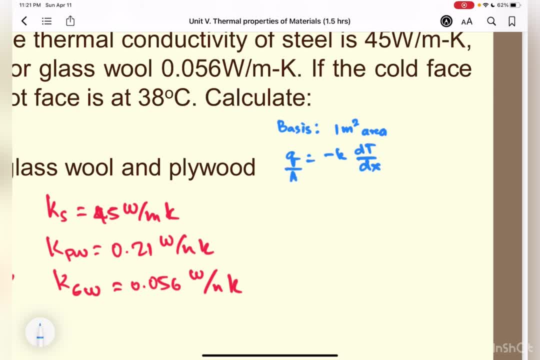 have your uh. this is q over a. sorry for that forward. or that is your. q is actually negative. ka, dt over dx. we define uh resistance to b, dx over ka, or, if i am, your resistance would be equivalent to delta X over K, a or Q. therefore, is D, T. 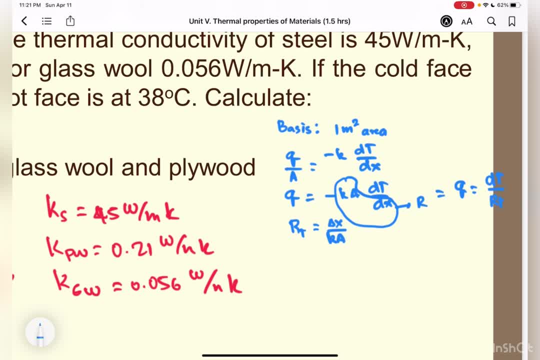 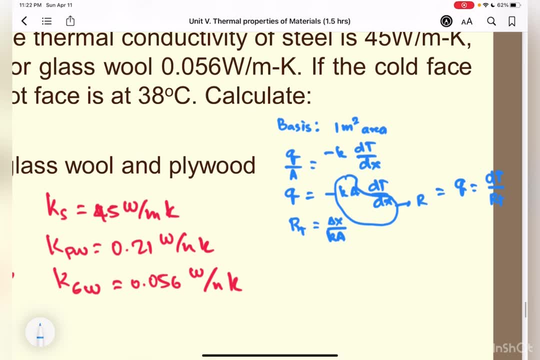 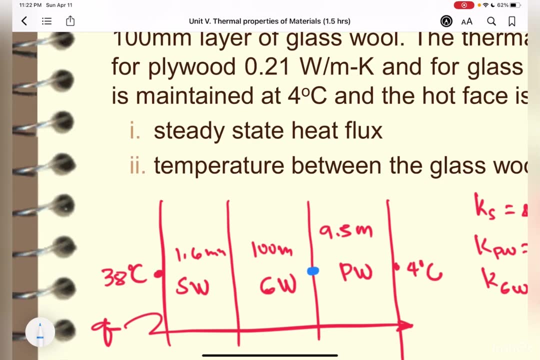 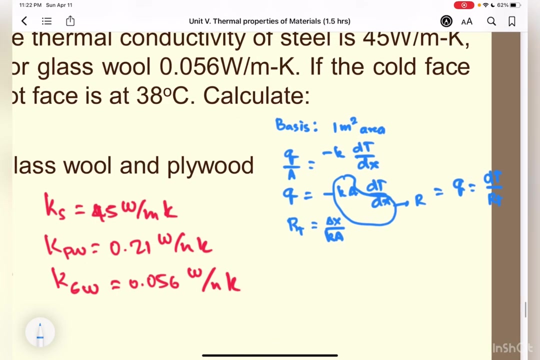 over R, the change in temperature over your resistance. okay, now let's take a look at the resistance. since it is, the wall is in series. therefore, resistance of the steel wall plus resistance of the glass wall plus resistance of your plywood would be your total resistance X. so that is resistance of the steel wall. 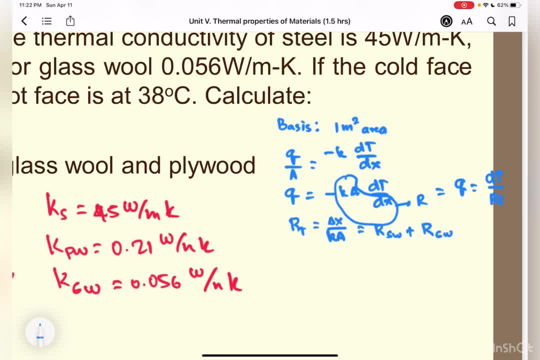 resistance of the glass wall plus the resistance of the plywood. okay, now let's take a look at the resistance. since it is, the wall is in series. therefore, resistance of the steel wall plus resistance of the glass wall plus resistance of your plywood would be your total resistance X. so that is resistance of the steel wall, resistance of the glass wall plus the resistance of the plywood. 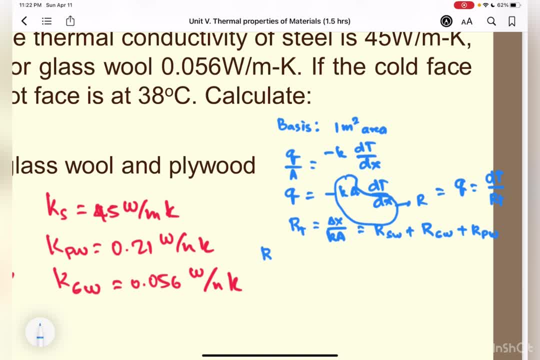 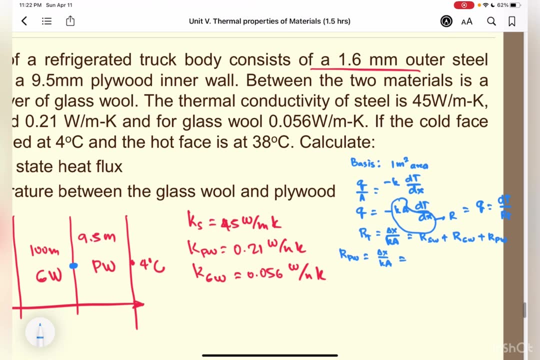 okay, let's take a look, find resistance of the plywood. first resistance of the plywood is Delta X over K. a. what's the Delta X change? it's nine point five millimeter, or that would be nine point five over one thousand to make it as a meter. K is point zero, point twenty one for the plywood, so it's point twenty one. 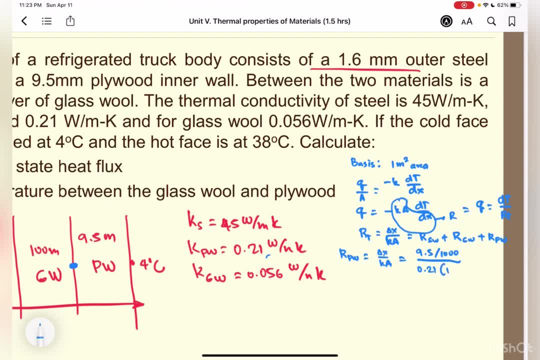 times a basis of your area of one meter square. so we got that to me around point zero, five for five two. okay, let's take a look at the resistance of the glass wall. last wall is one hundred millimeters, so one hundred over one thousand divided by K, of the glass wall which. 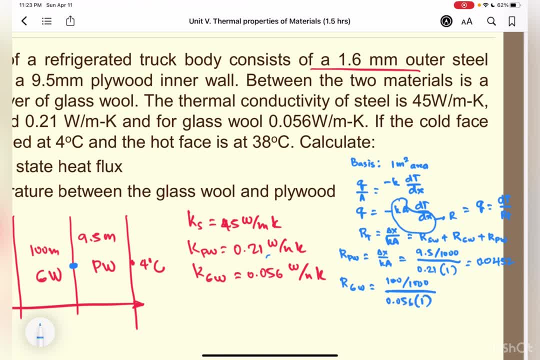 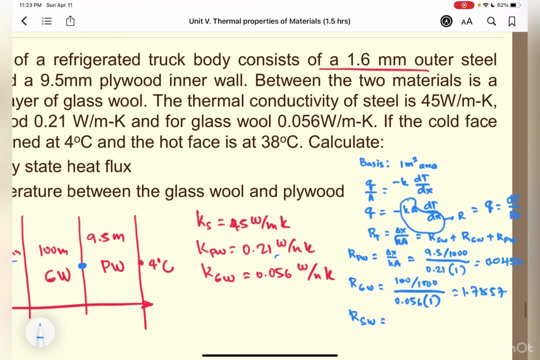 which is 0.056 times 1, that's around 1.7857. lastly, resistance of the steel wall. i have 1.6 millimeters, 1.6 over 1000 millimeter per meter times the k is 45 times the basis of. 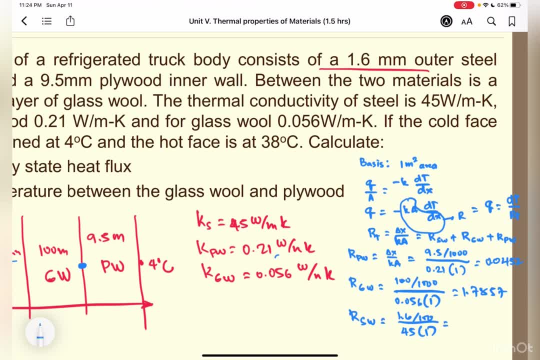 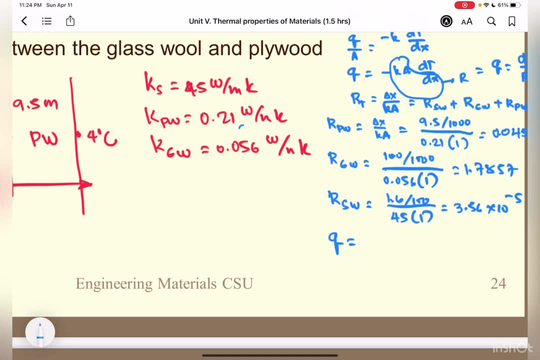 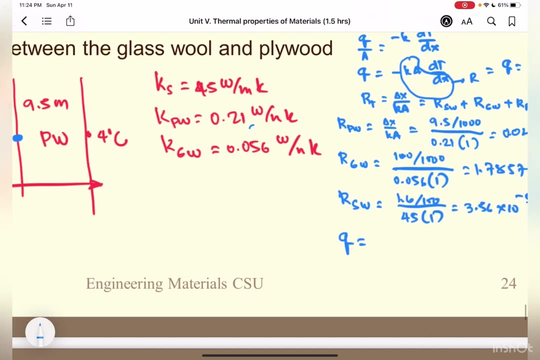 one meter squared, you get that as your 3.56 times 10 to the negative five. knowing all the resistances, i could now get my q that this q is the delta t, the change in temperature from 38 to 4, which is around 34 degrees, divided by the total resistances. 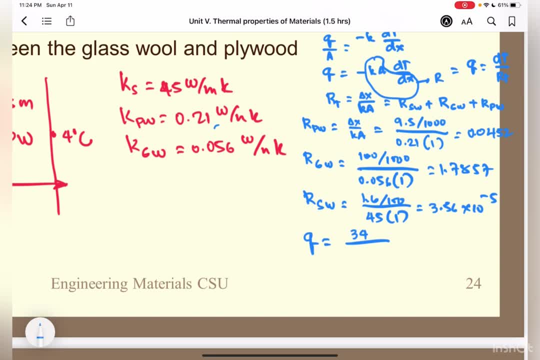 you get that as your 3.56 times 10. to the negative 5, knowing all the resistances, i could you add 0.0452 plus 1.78 plus 3.56, so that's around 1.831 and you can get this to be 18.57. 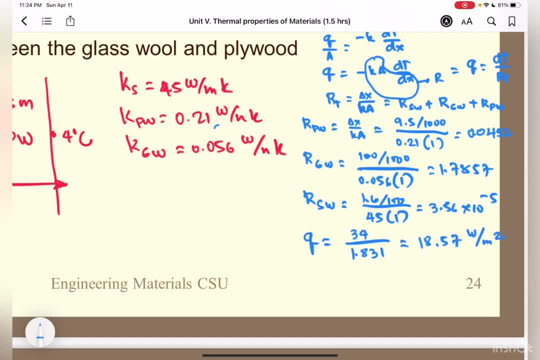 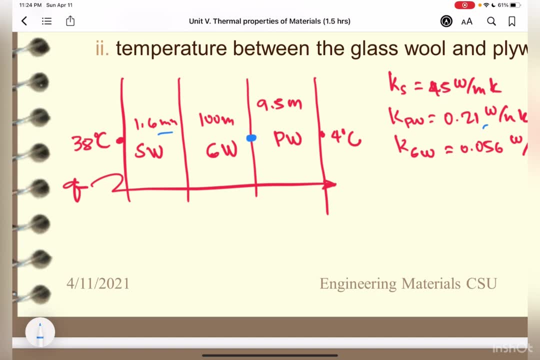 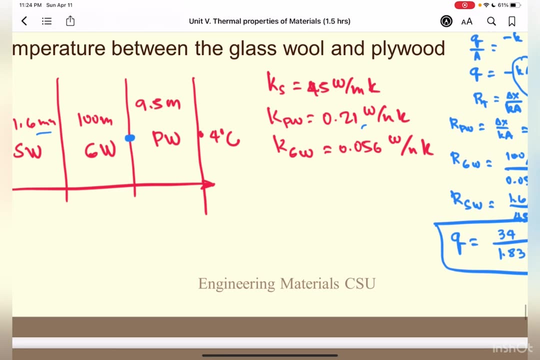 watt per meter squared. so this would be your q, since it is in series. whatever is the heat transferred along the steel wall, it would just be the same with the glass wall and the plywood. so i could use your q in getting the temperature between the two insulators. 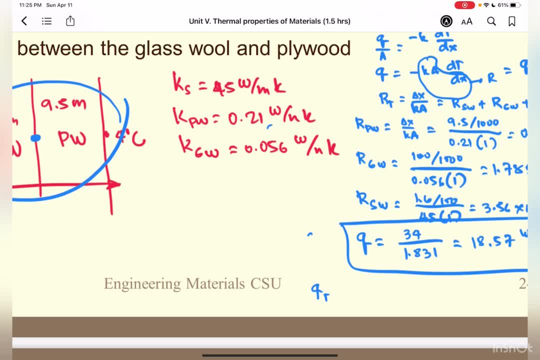 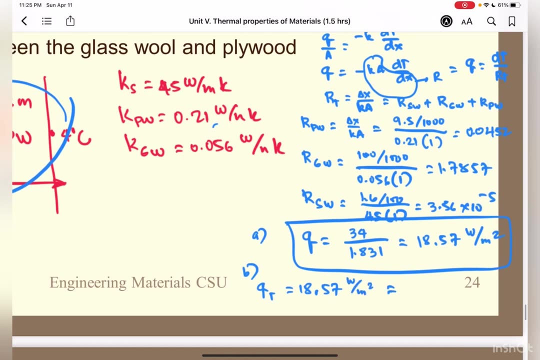 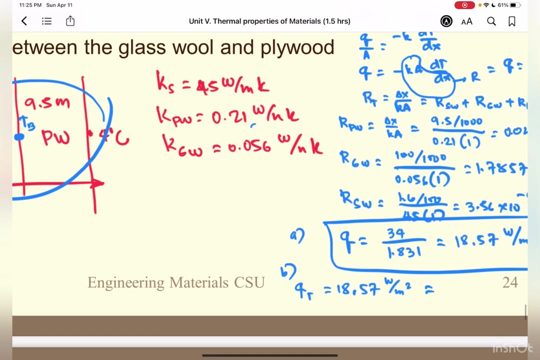 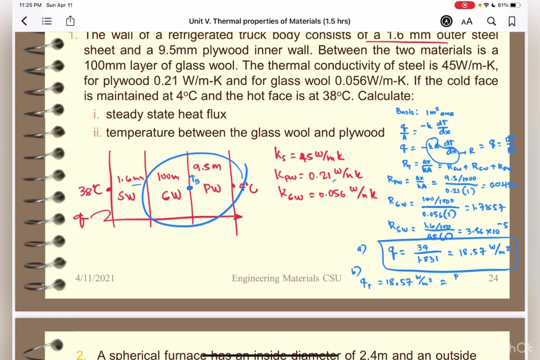 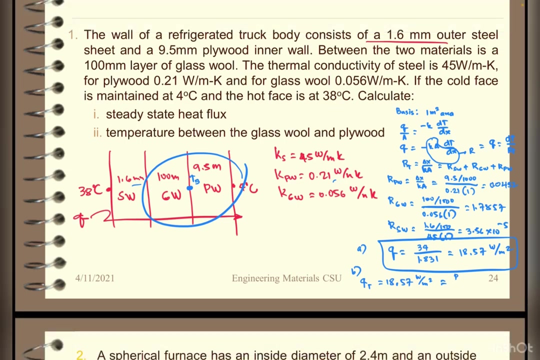 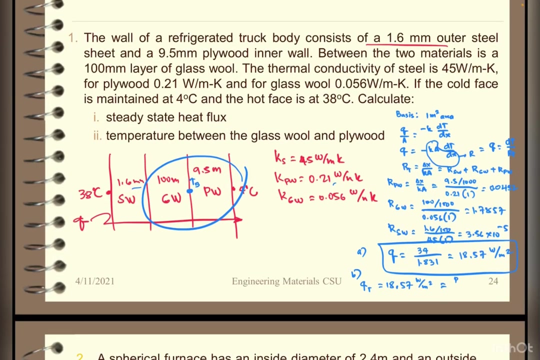 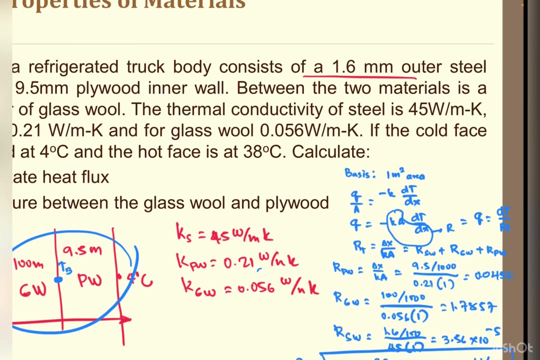 or that. your q total, therefore, which is 18.57 watt per meter squared. that is actually equivalent to the change in temperature, assuming that this is tb. so it is tb minus four degrees. so you have here tb. what happened to my dl? all over the resistance of your plywood? 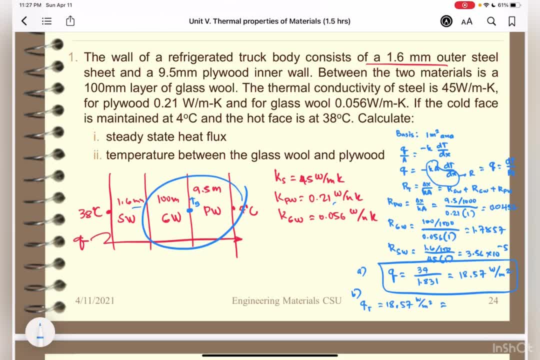 and computer, for your db, you get to be claiming, and you will see that here. you will see that here. this solution for reading電, for for the clapboard and for the ambled- yes, this is still the same. okay, so here's Outside: four point TB would be around four point eighty four degrees Celsius. okay now. 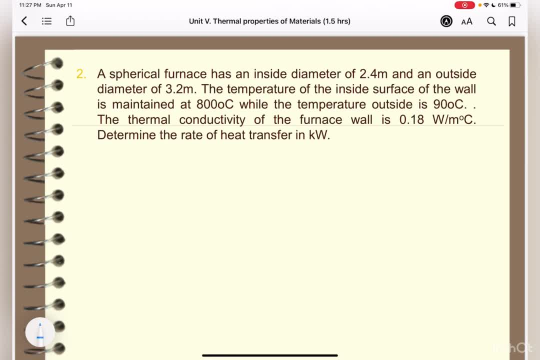 let's proceed with another example. say, I have a spherical furnace which has an inside diameter of 2.4 meters and an outside diameter of 3.2 meters. the temperature of the inside surface of the wall is maintained at 800 degrees C, while the temperature outside is 90 degrees centigrade. the thermal 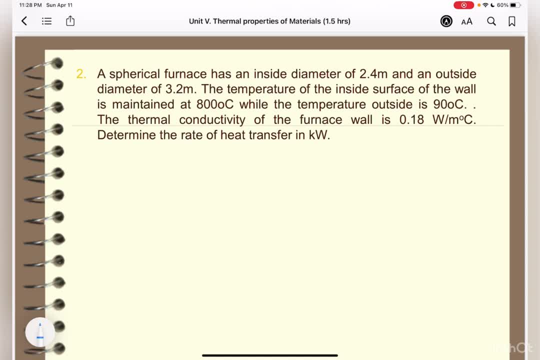 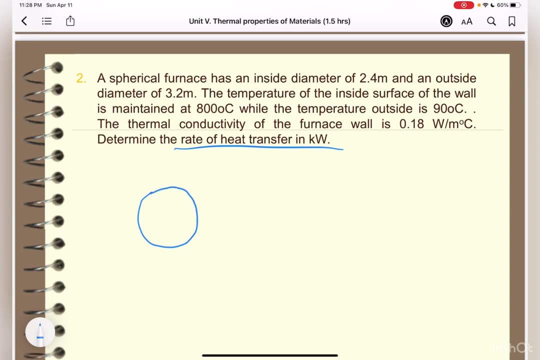 conductivity of the furnace wall is given as point eighteen watt per meter degrees Celsius, we're tasked to get the rate heat transfer in kilowatt. okay, so, assuming you have just to show you the inside and the outside diameter, okay, inside diameter is given us 2.4 meter, while that of the outside I have here dead amorous I. 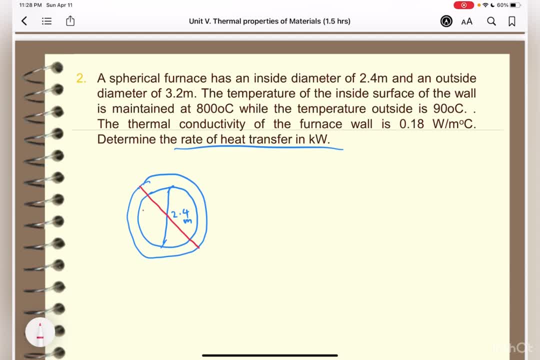 diameter is three point two meters. okay, the inside wall here is maintained at 800 degrees c, while that outside is at 90 degrees centigrade. now it has to get the rate of heat transfer, of course, from the inner going to the outer. so, assuming this would be the q that we are looking for, okay, 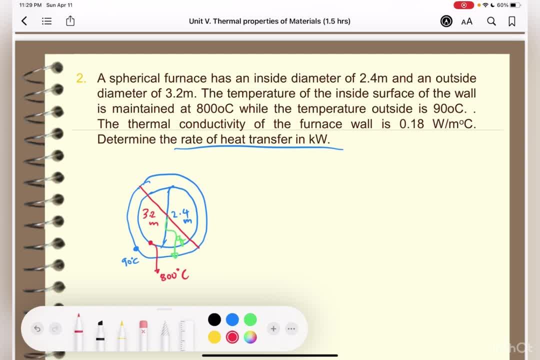 then we have from our equation: q is equal to delta t over rt. order your resistance so we could get that easily as negative 90 minus 800, all over the resistance of what's your delta x. we need to get the delta x here and also the area. so the area actually is four pi. so since it is uh sphere, four pi, r, one, r, two. 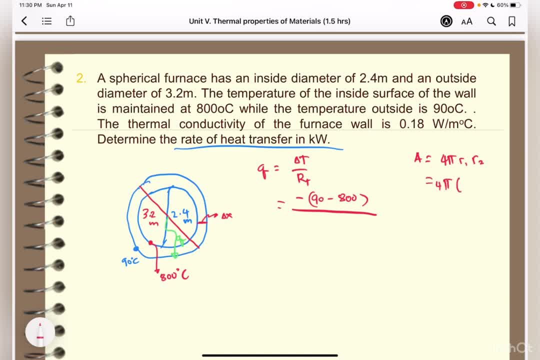 or that is four pi times two point, two times two point four. okay, so that's roughly 12, 24 point, i think, 24 point uh 13.. so if it is 24.13, i could now plug it in my equation that your rt is delta x over ka. 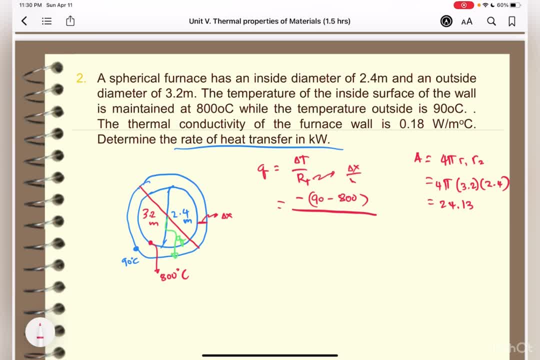 right, this one, it's delta x over k. a delta x is this one: it's 3.2 minus, uh, 2.4 divided by 2. okay, so if it is, delta x is 3.2 minus 2.4 over 2, so you get your delta x to be around 0.4. so divided by 0.4 over k, given k as 0.18. 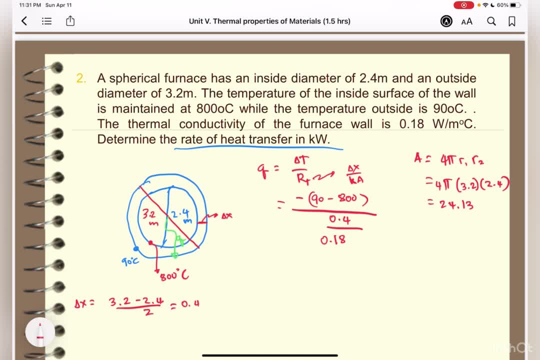 times the area of 24 point rating. so you get easily your q to be roughly around 7.71 kilowatt now, without actually knowing your fourier equation, you could, you could, uh, use your differential equation, uh formula. how is that? you know for a fact that your q is actually negative? k, a dt over dx or q would be the integral. 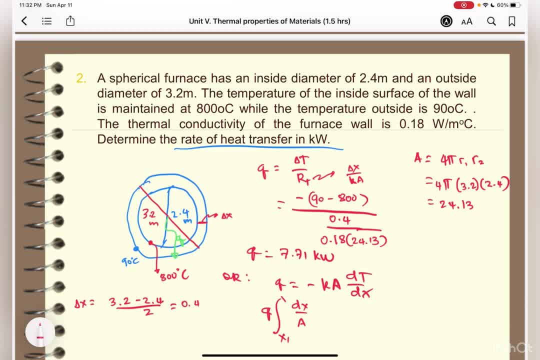 of your dx over a, from your x1 to x2 and this is negative integral, from t1 to t2 of your dt times, k or k b t. now, if you know this one, you have here, your four q is equivalent to uh integral from- sorry for that, okay, q4. so this is dx over a. you know that this is d1 over d2 is. 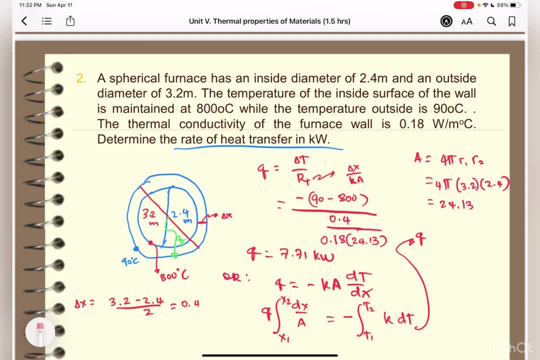 going to give us playing with a integral from a and a to gratuitously from a and dN, from a, because you know that this is from radius is 1.1 to 2.4 diameter, so that's 1.2 to 3.2, that's 1.6 in terms of radius dr over. 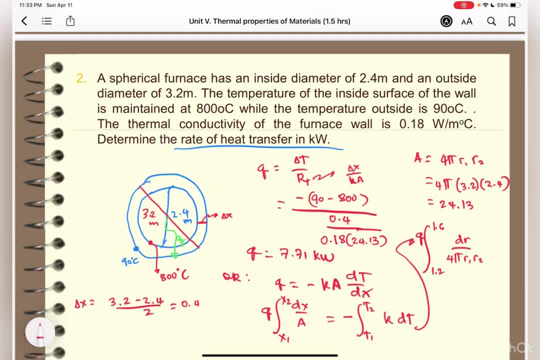 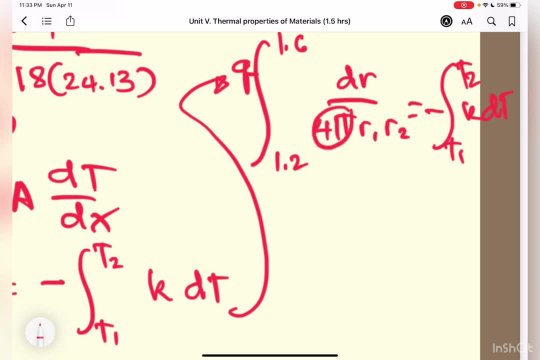 4 pi, r1, r2. it's equivalent to same t1 to t2, negative k, dt or these are constants. i could i could bring that out. so i have q over 4 pi integral from 1.2 to 1.6. derivative of dr. 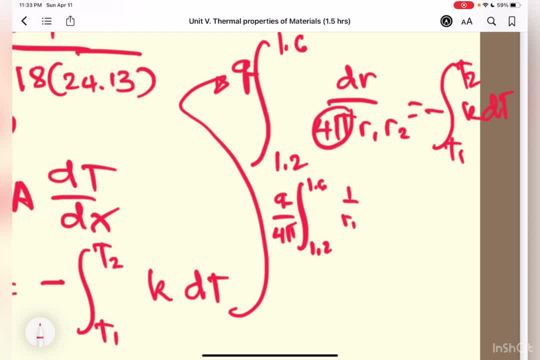 over 4 pi. r1, r2. it's equivalent to same t1 to t2, negative k, dt or these are constants, so i could i over r1. r2 is equivalent to 1 over r1 minus 1 over r2. okay, it's equivalent to negative 0.18. 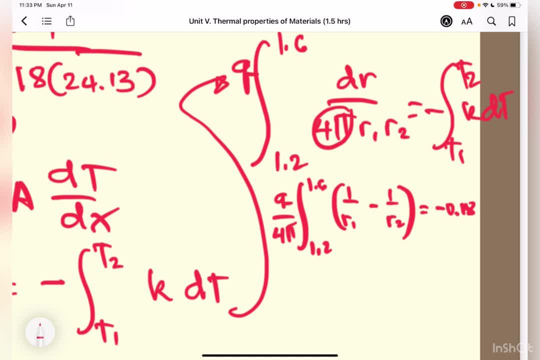 that's your k, and derivative of dt from t1 to t2 is t2 minus t1 or 90 minus 800. so you have here therefore, q over 4 pi times 1 over 1.2 minus 1 over 1.6 is equal to negative 0.18 times 90, or, if i 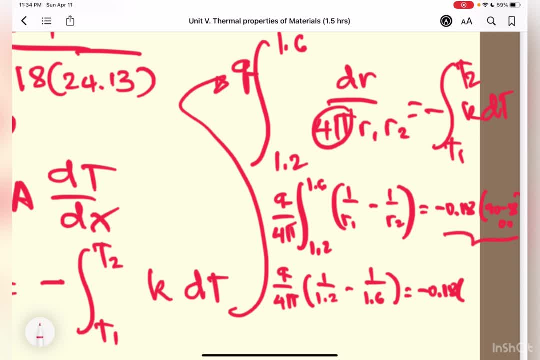 get the value of this, it would just be equivalent to negative 0.18 times 90. or if i get the value of this, it would just be equivalent to negative 0.18 to 127.8. and finally you could get q to be 127.8 times 4 pi all over 1 over 1.2, minus 1 over 1.6. 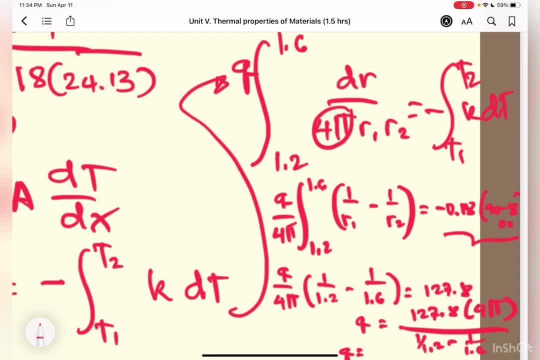 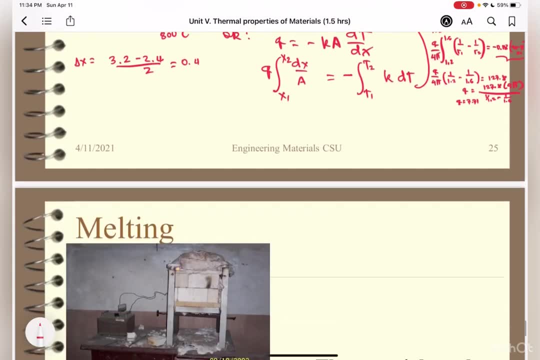 and you'll find it to be equivalent also to 7.71 kilowatt. okay, so that is the answer to this question. so if you have any questions, please feel free to ask me in the comments below. that ends our uh or not yet. so i still have here some figures about melting. so this is actually. 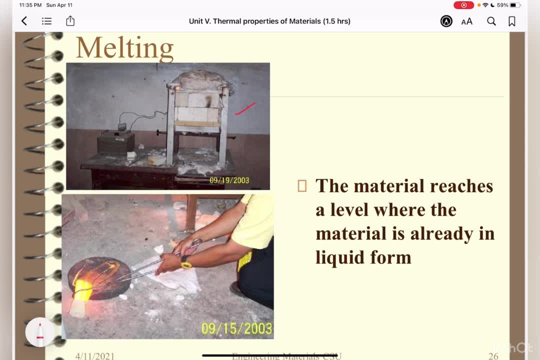 a kiln or a small furnace in msdd osd, wherein we have here a ceramics that is being subjected to as high as 1200 degrees celsius and then the material would reach a level that is already. it becomes liquid form. you can just pour it out, okay.